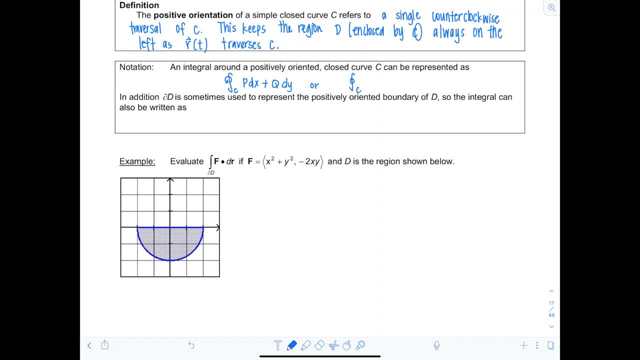 in such that that都有 R when we use this倒 is positive. So in addition, sometimes you'll see Delta of capital D And that can be used to represent the positively oriented boundary of D. So this same integral could also be. 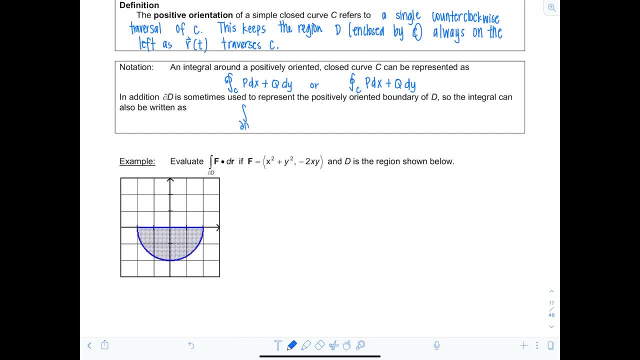 written as follows. So you could have the integral over Del capital, D representing the, which is that closed curve, p dx plus q dy. So they all mean the same thing. I just want you to be familiar, depending on whatever you happen to see. All right, so let's look at an example here. 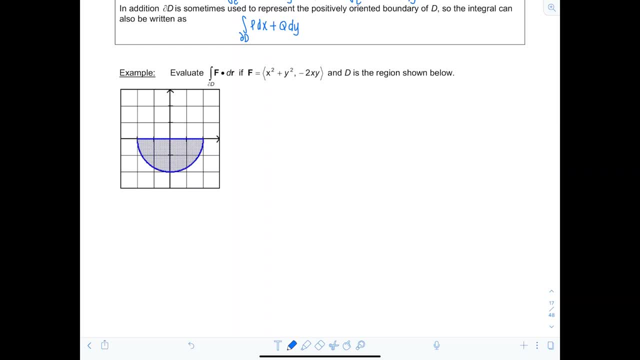 Evaluate the following line integral. remember this represents work if we have the following vector: field f with components x squared plus y squared, so that's p and here's q. Now, remember, we just learned the fundamental theorem for line integrals, which tells us that 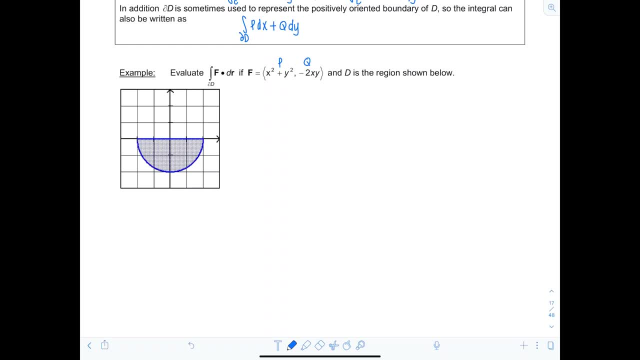 if we have a conservative vector field, then we are able to use the fact that the work on any closed curve is going to be equal to zero, since we just take the potential function evaluated at the end point minus potential function at the initial point, and if it's a closed curve, those 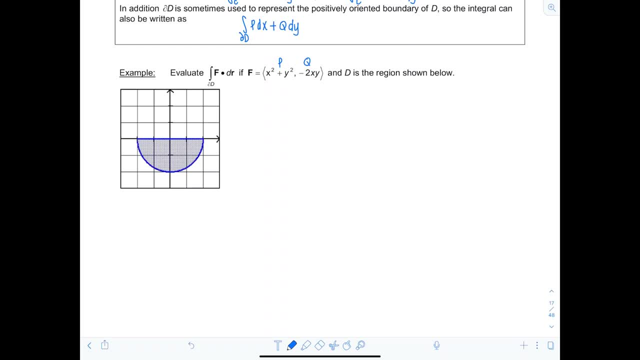 are going to be the same. If you need a review, you can go back to the previous video, But that only works if your vector field is conservative and in this case, notice, it's not. How do we check again? Well, remember there's three conditions. 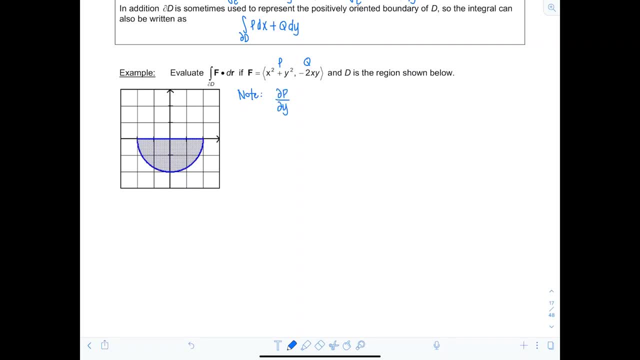 the first being that those mixed partials have to be equal. So del p del y, that's equal to 2y, which is not equal to del q del x. What's del q del x? It's negative 2y. So this is not a. 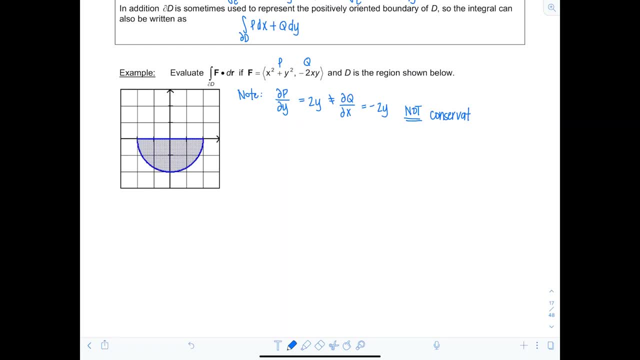 conservative vector field. I could not find a potential function whose gradient this vector field would be, So I do want to find a function whose gradient this vector field would be. So I do want to find a function whose gradient this vector field would be. So I do want to find a. 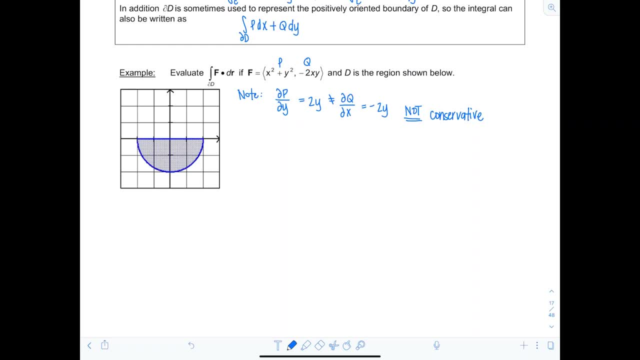 function whose gradient this vector field would be. So I do have to compute this line integral directly for now. So what I need to do is first parametrize this curve And notice I have to do it into two pieces. So standard orientation, positive orientation, would be counterclockwise. 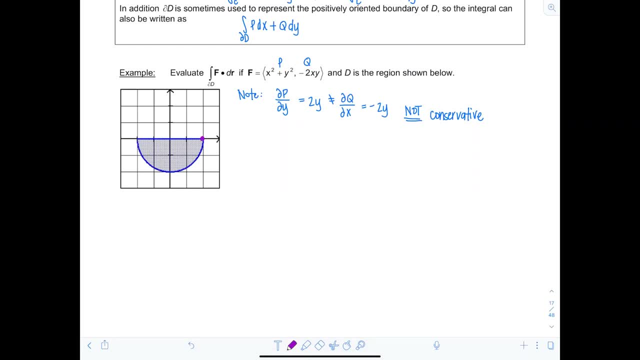 So we'll take the portion starting from 2020 at negative two zero. that's going to be C one, my first curve, And then the second portion is going to be that bottom half of the circle. and remember we always have to go counterclockwise unless directed otherwise. okay. 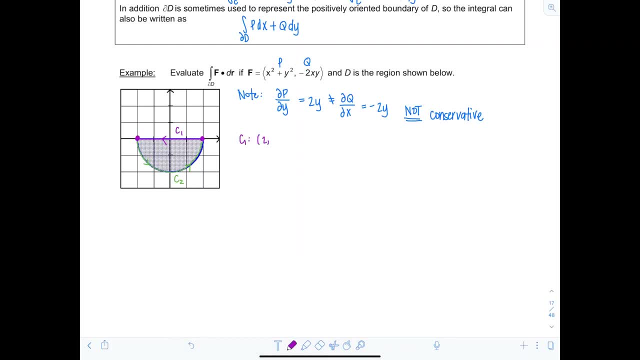 so my first curve is the line segment from 2: 0 to negative 2: 0. alright, so remember your parameter has to always be increasing, so you can't define it backwards just because you want it to start at 2 and end at negative 2. T has to go between negative 2 and 2, so what do you do to compensate? 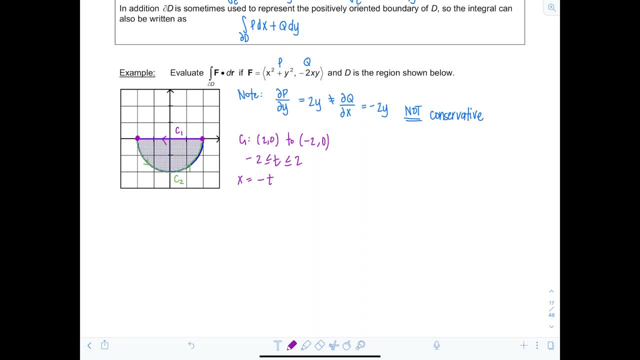 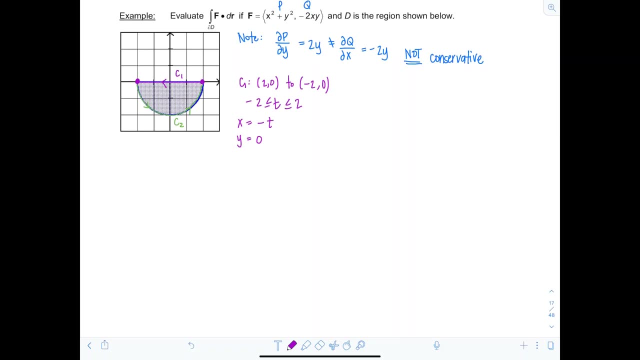 well, you say X is gonna equal the opposite of T, BAM, then you're okay, and then Y is equal to 0. so there's our parameterization. since I know I need PDX plus Q, D, Y, let's go ahead and find DX and dy right now. so DX would be negative, D, T and then dy would just be 0, okay. so that's for the first. 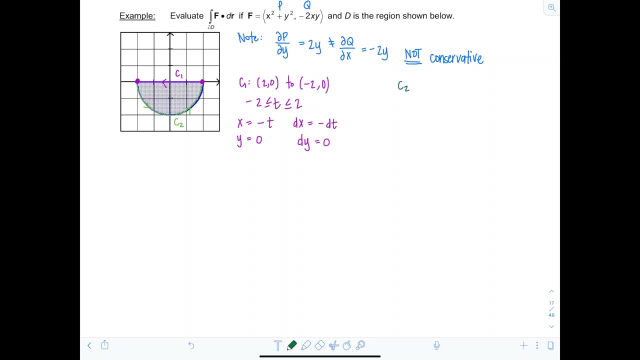 curve. now what about the second one? so I need the lower half of a circle centered at the origin. radius is 2 and we're going counterclockwise. so perfect X is going to be 2 cosine of T and then Y is going to equal 2 sine. 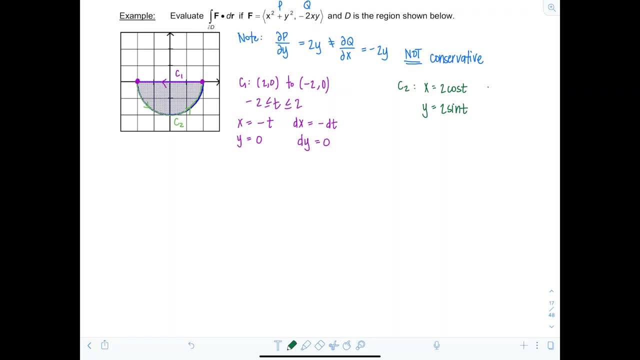 T. and then let's get DX and dy. so DX would be negative 2 sine, TDT, and then dy, 2 cosine of T, DT. and then what should the limits be for T? you have a couple options. I'll just do from P Eye to 2 Pye. I'll turn it to me. you could go negative pie to 0 if you prefer. okay, very good. so now we're. 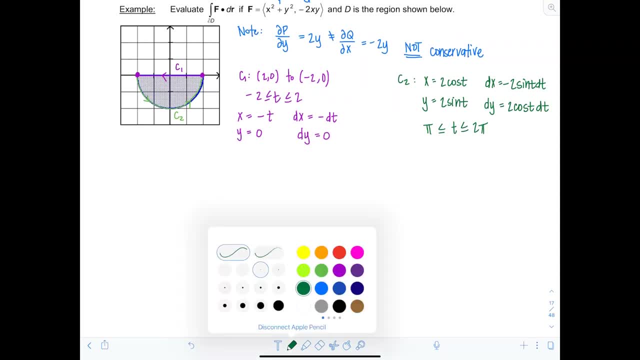 all set up. in order to compute this integral, I'm gonna have to sum up the line integral over curve 1 and curve 2, right? so I'm gonna, girlibel, be for this original circle here and it needs 1 over Q, 2 plus C, X plus Q inside this integral, which is 2 elephant on X and humiliate stacked values of. 0 d and sorry for a little kid later. thanksı did all of them do the work. so now this integral is the into D. D is done, so that's the next step. I'm going to have to sum up the line integral over curve 1 and curve 2, right, so I'm going to do this. 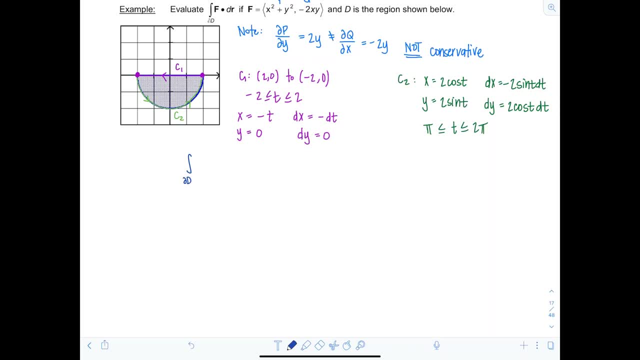 process of duas times to the middle right and then connect it to the podemos del a plus c line integral for del d for this closed curve of f dot dr is equal to the line integral over c1 of f dot dr plus the line integral over c2 of f dot dr. 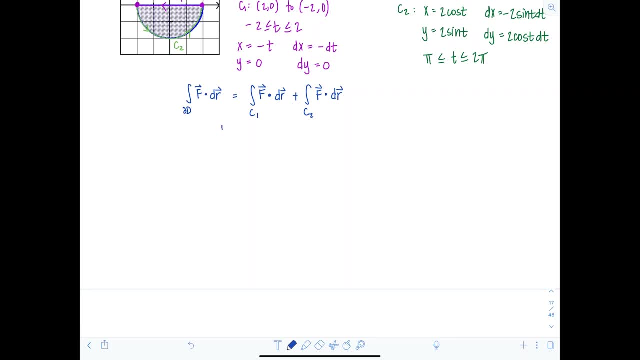 All right, so we'll just use pdx plus qdy, First line integral over c1, the limits of integration are going to be from negative 2 to 2, because- notice, that's what my limits were for t- here I need pdx. Well, where's p? P is x squared plus y squared, but remember: 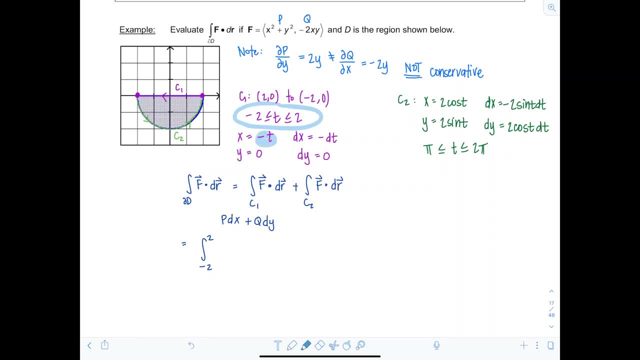 on that curve. I'm letting x equal negative t and y is zero. So x squared plus y squared is 0.. So x squared plus y squared equals 0.. So this is 1.. So this is 1.. And then the Christina Hatch. 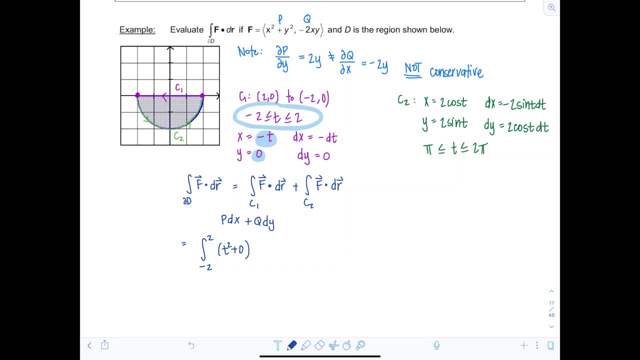 squared is going to be t squared plus 0.. And then dx is negative. dt plus qdy, That's just going to be 0.. Plus, now let's move on to curve 2.. Now the limits of integration are going to be from pi to. 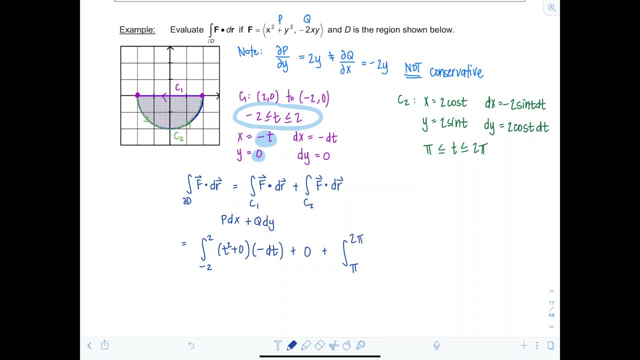 2 pi, p, dx. Well, I'm going to have, let's see here: p is x squared plus y squared. Well, square this, that's 4, cosine squared t. Square this, that's 4, sine squared t. Add them up, that's 4.. So that's p. 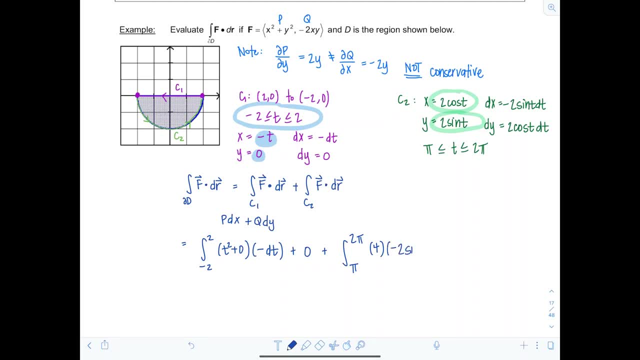 dx is negative 2 sine t dt plus q is negative 2xy. All right, So negative 2 times 2 cosine t y is 2 sine t. And then I need dy, which is going to be 2 cosine t dt. So let's scoot over, scoot, scoot. 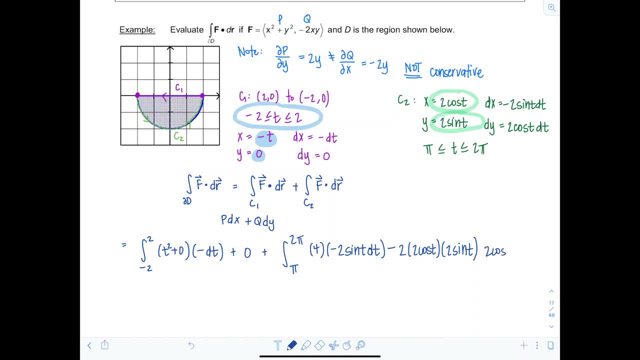 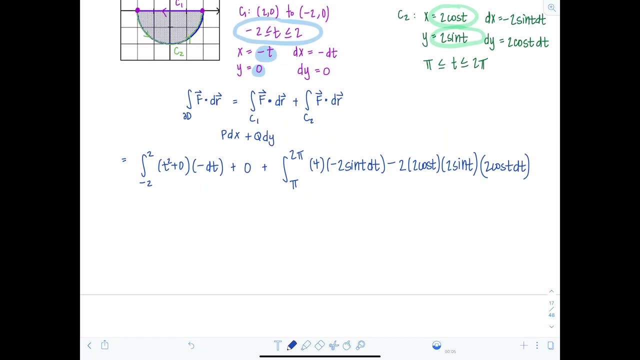 And then dy is 2 cosine t dt. All right, So now everything's in terms of t. Let's go through see how we would anti-differentiate. So first integral, that's easy. Just take the negative outside. Then you have negative 2 to 2, t squared dt- beautiful. 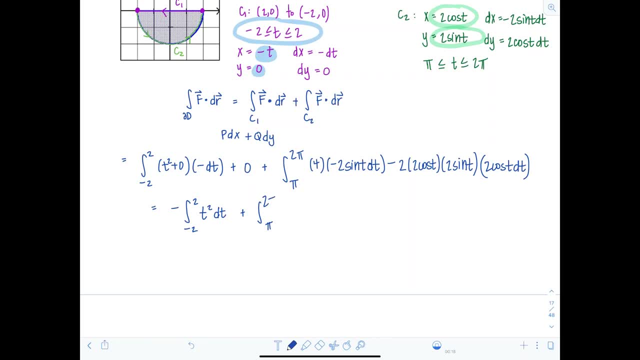 Plus, let's see here I have pi to 2 pi. This first term here is going to be negative 8 sine t, And then I'm going to have a cosine squared t, a sine t and 2 times, 2 times 2,. 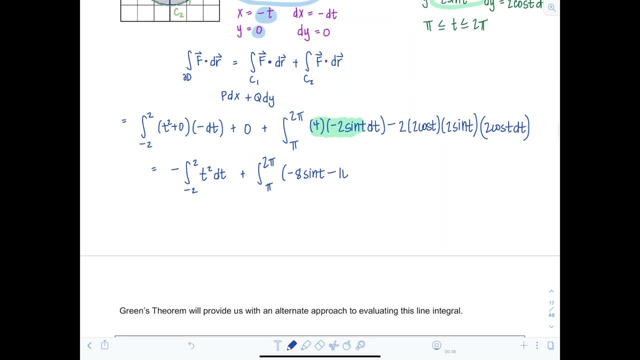 so that's 16, cosine squared: t, sine t, dt. All right, Now from here, what would you do? Well, let's see, Let me make this look beautiful. Okay, t squared, we got it. Sine t, we got it. And then for this, cosine squared in your head. 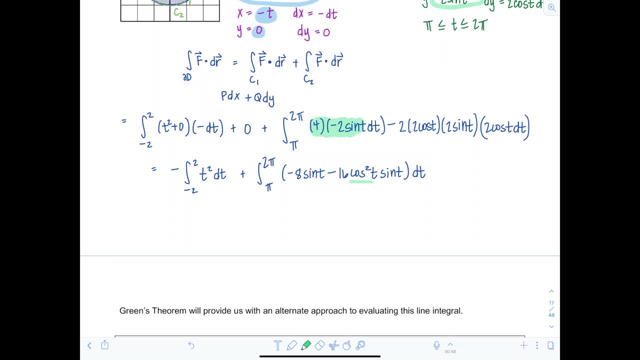 just let u equal. cosine t du would be negative, Sine t dt, but that's okay, You already got that negative, So you would just have to divide by 3,. make it a cosine cubed, call it a day. All right, Not too bad, You guys can work that out pretty. 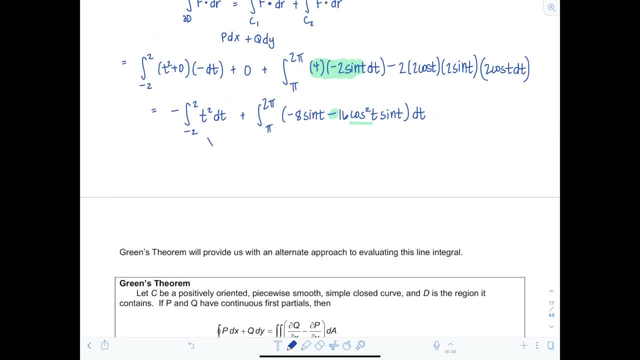 easily. So the first integral is going to give you a negative 16 thirds Plus. then you should get 80 thirds from the second integral And putting it together that gives you 64 thirds. All right, So not too bad right. That was pretty manageable. 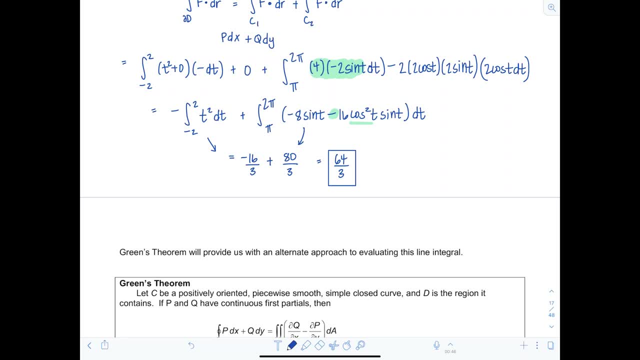 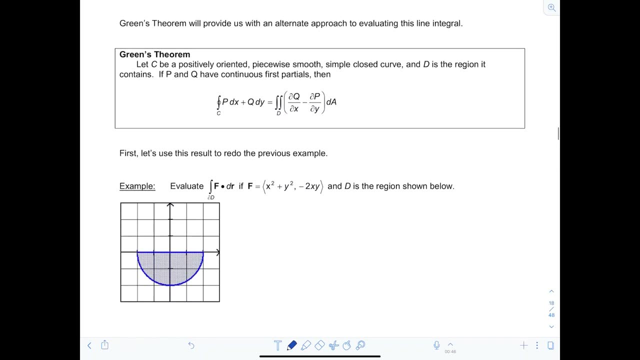 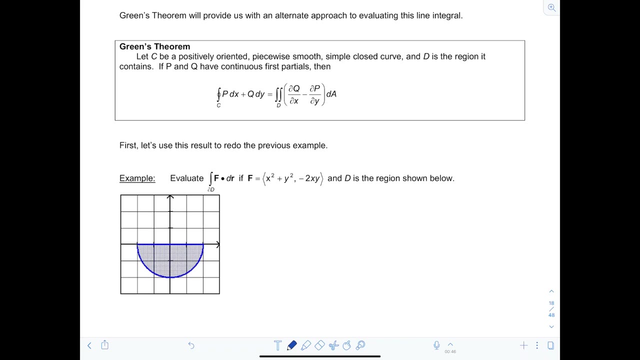 Now let's see what Green's theorem says and how we could apply it to the same example. All right, Now Green's theorem is going to provide us with an alternate approach to evaluating this line integral, and it states the following: So let c be a positively oriented, piecewise, smooth. 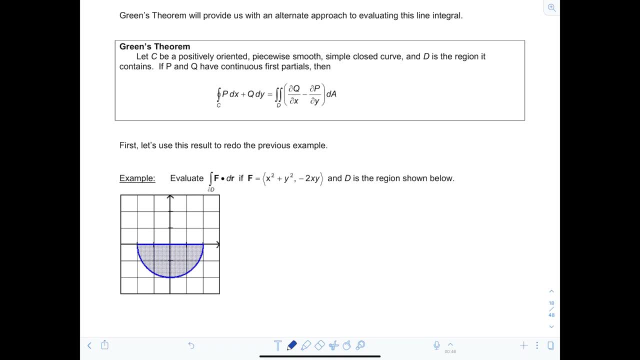 simple closed curve and d is the region it contains. Okay, Got it. If p and q have continuous first partials, then- And remember this integral represents work. Okay, The line integral over the closed curve of pdx plus qdy is equal to the double integral over the region d. 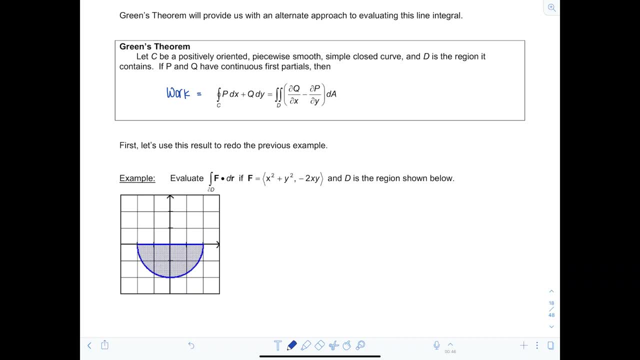 of del q del x minus del p del y, dA, All right, And then you can see if your vector field is conservative. we know del q del x has to equal del p del y, And so this quantity would be zero, right? So the work on the vector field is. 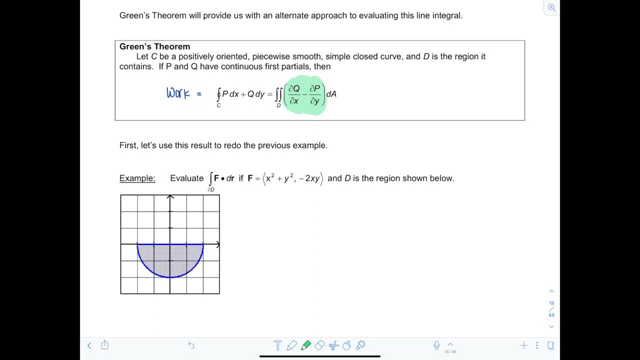 going to be zero as long as you have a conservative vector field. So you would only need to compute this line integral if you don't have a conservative vector field. Okay, Before we prove Green's theorem, let's use this result to redo the previous example. Okay, So we want to evaluate the work. 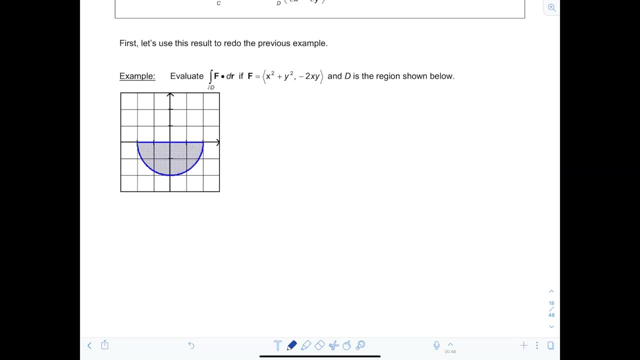 for the given vector field. and this time I'm going to apply Green's theorem And you might think: oh no, I don't want to do a double integral, Yes, you do. Okay, It's going to be a lot nicer most of the time. So let's figure out double integral over the region d. 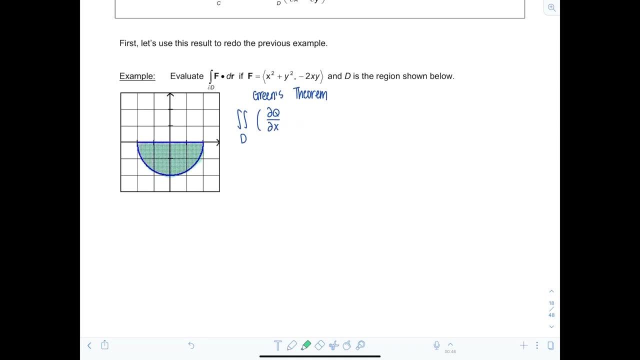 So d being this region enclosed by that closed curve, minus del p del y, dA. Okay, So this is going to be double integral over d del q del x, that's negative 2y del p del y, And then we're going to compute the work over this region d by the closed curve. 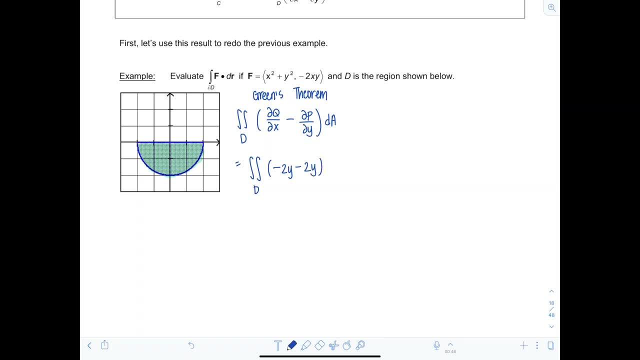 that's 2i, so minus 2y da. so I can clean this up. I can take out a negative 4. I have double integral over d of y da. now it makes sense here to go polar right, so I'm going to write this as negative 4. 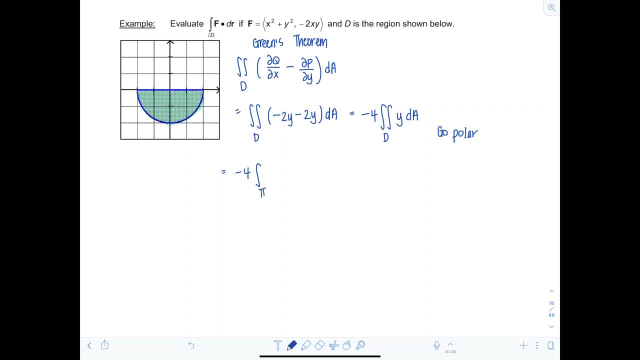 times the integral limits for theta should be pi to 2 pi, and then limits for r should be from 0 to 2. and then, remember, I have to replace y so that it's in terms of polar coordinates, so r sine theta. and then da is, you guessed it, r dr d theta. 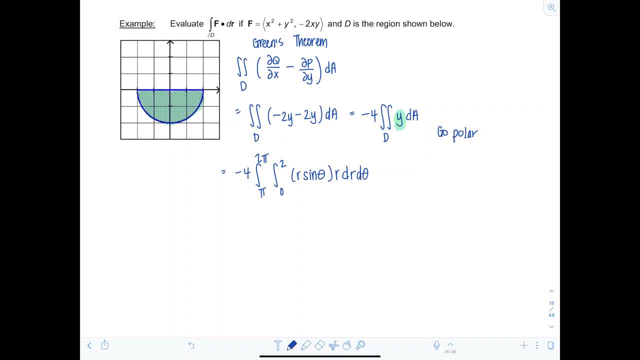 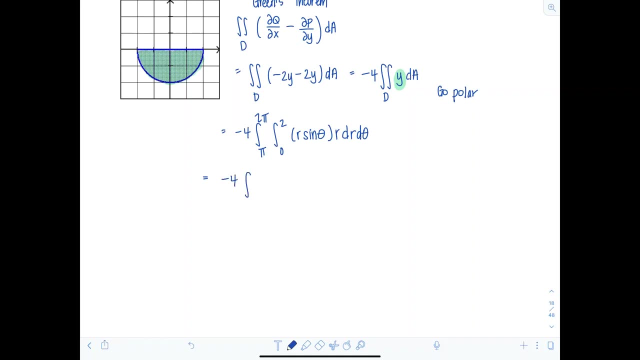 okay, very good, so I can rewrite this as a negative: 4 times the integral from pi to 2, pi of sine, of theta, d, theta times the integral from 0 to 2 of r squared dr. And lo and behold, this is going to give us 64 thirds, just like we got. 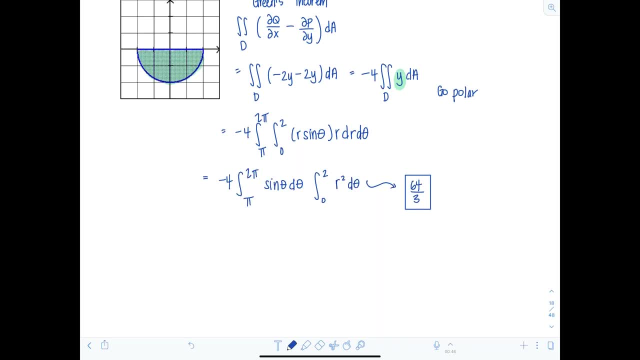 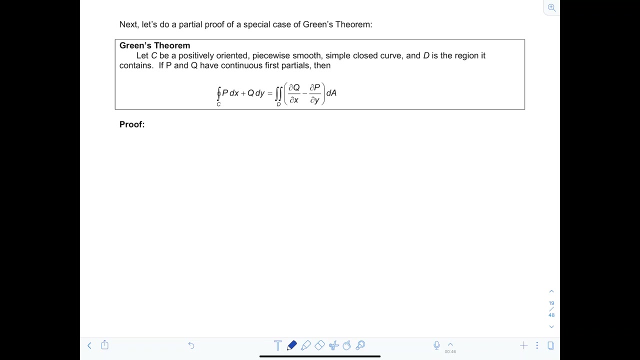 before Now I told you we were going to prove Green's theorem. We're going to do a partial proof of a special case, because the complete proof is rather involved. So we're just going to look at one special case and just partially prove it. Okay, so here's Green's theorem stated. 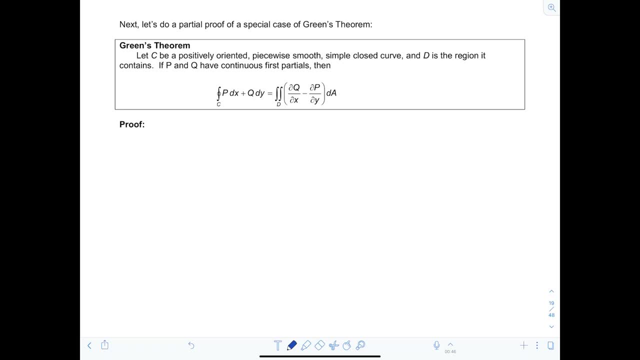 again, And what we need to do in order to start this special case is make some assumptions. Okay, so I'm first going to suppose that the region D is both type 1 and type 2.. What do I mean by that? Well, remember, we classified regions type 1, type 2, if it can be. 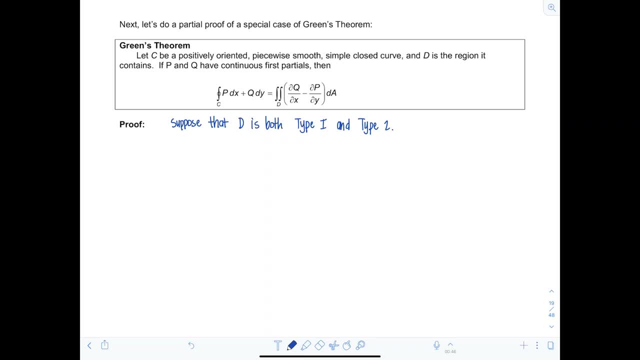 bounded in the y-direction or bounded in the x-direction when we were finding areas between curves or areas of regions. So I'm assuming that this region D- I could express it either way- Okay, so if I can show that the region D is both type 1 and type 2, then I'm assuming that the region D is both type 1 and type 2.. 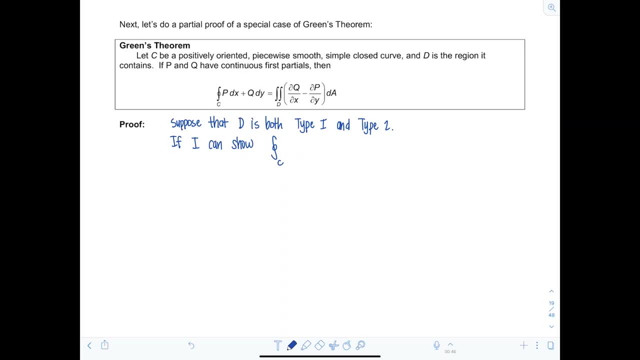 Okay, so if I can show that the region D is both type 1 and type 2, then I'm assuming that the region D is both type 1 and type 2.. Then I'm assuming that the line integral over C, the closed curve C of PdX, is equal to the double integral over D of negative del P del y. 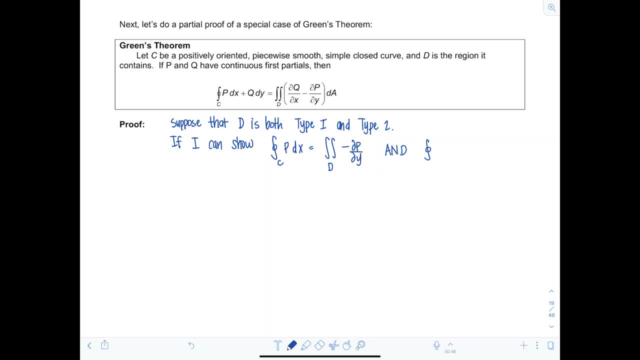 And if I can show that the line integral over our closed curve C of QdY is equal to the double integral over D of del Q del x' dA- Oops, I forgot the DA here, Excuse me- Then adding those two equations together. 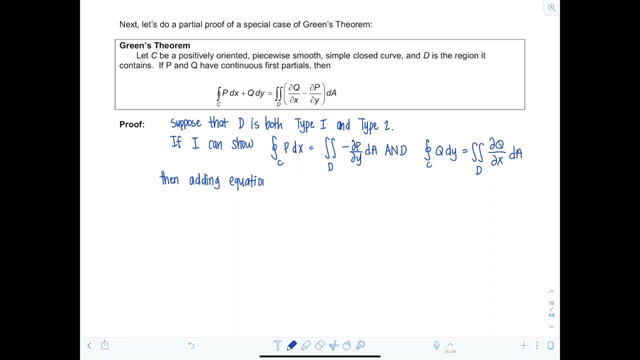 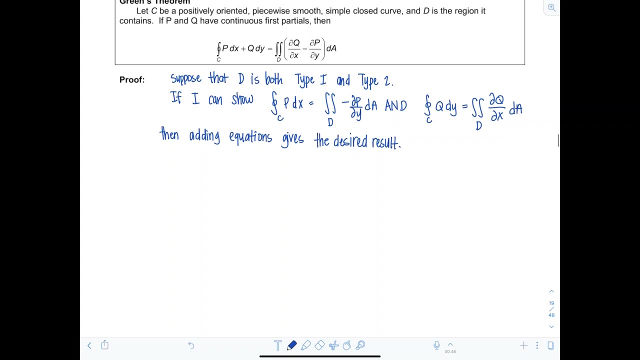 gives the desired result. Okay So I'm going to focus on showing this first equality right now. Okay So let's focus right now on P And I'm going to draw the region D right now In a special way. Okay So I'm going to say here's a curve And then here's another curve. 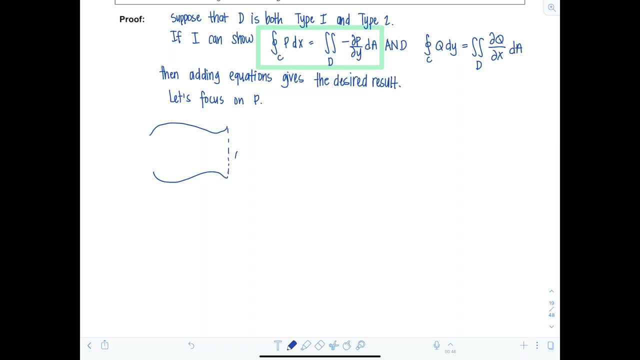 Remember we have to go counterclockwise And these are the limits. So this is X equals B, This is X equals A. Here's my curve. So G sub 1 of X And this is G sub 2 of X. these 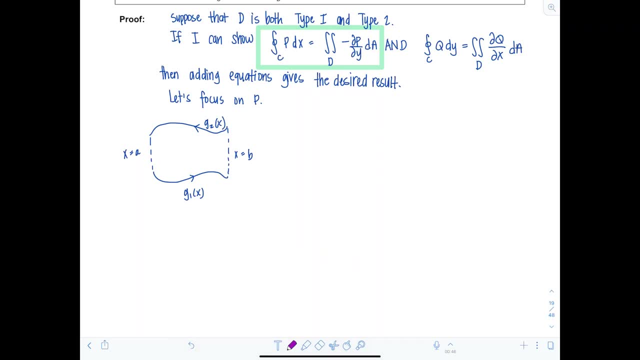 curves. And then here's my region D. inside here This is D And I'll call this curve C1. And then this one up here is C2.. Okay, So let's consider the line integral around the region for the closed curve C of just PDX. Okay, 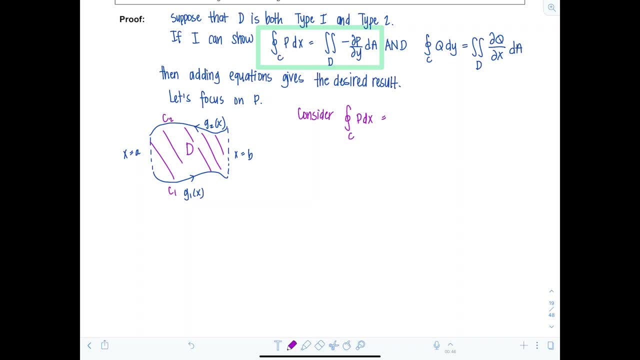 Now I can notice I wrote C as the sum of C1 and C2.. So I could write the integral similarly As the sum of C1 of PXYDX plus line integral over C2 of PXYDX. All right, Well, in this particular case, yeah, I can write Y as a function of X. So 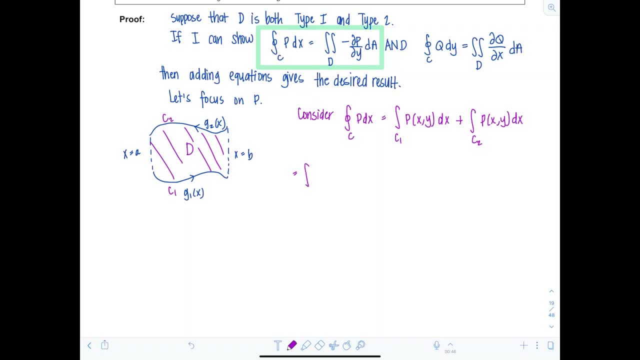 on the first line, integral. I can write this in terms of X, everything, So limits are from A to B. I would have P of X, And then, instead of Y, I'm going to write G sub 1 of X, because that's how Y is defined. 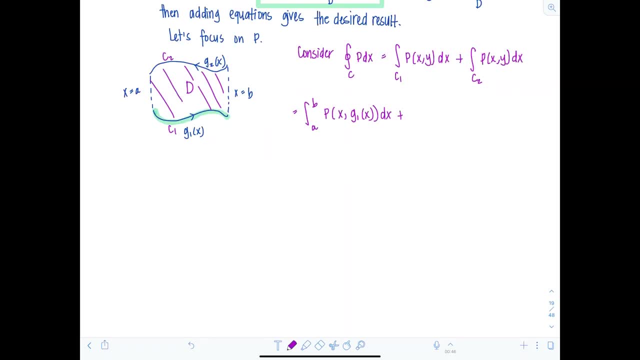 on that first curve And then for the second line, integral notice, the limits are going to go from B to A, And then I have P of X And then Y is equal to G sub 2 of X- DX. Okay, If I want to combine the integrands, I just need to flip the limits of integration. 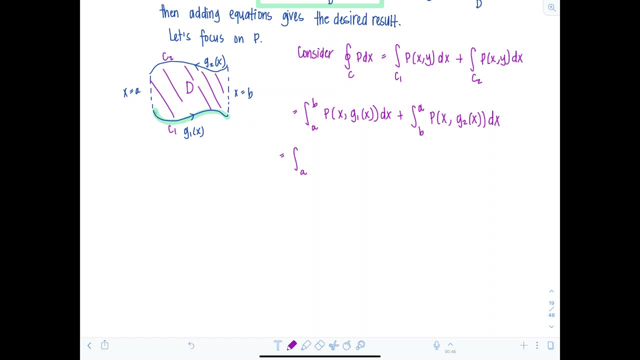 on the second integral. So that's fine. So I can write it as the integral from A to B of P of X G, sub 1 of X, minus P of X G, sub 2 of X DX. Okay, Looks good, We're going to put this on hold now. Okay, You know, when you watch a cooking show, 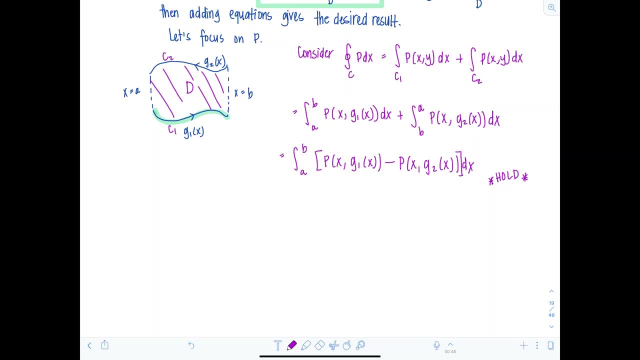 and they've got something and they're like we're putting it on the back burner to simmer. Well, I work on some other dish that needs to get started. That's what we're doing. Okay, Now I want you to consider: 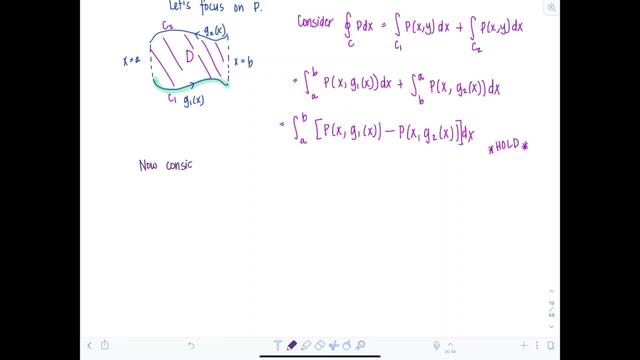 a double integral. We're going to consider the double integral over that region D del P, del Y, DA. Okay, Well, I said that this could be a type 1 or type 2 region, meaning I can express it with constant limits in terms of X. 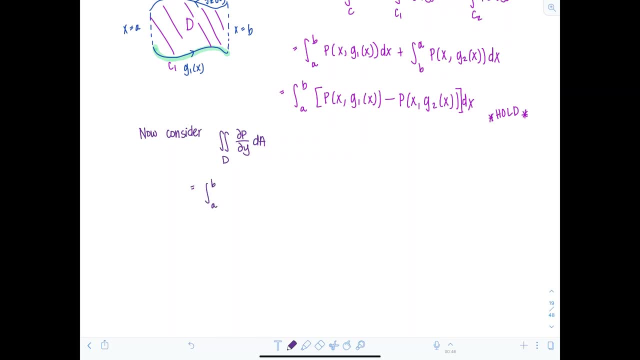 or Y just as easily. So say, we have constant limits for X on the outside Limits for Y, lower limit would be G sub 1 of X, Upper limit would be G sub 2 of X, del P, del Y, And then, in this case, DA I've chosen the order to be DY, DX. 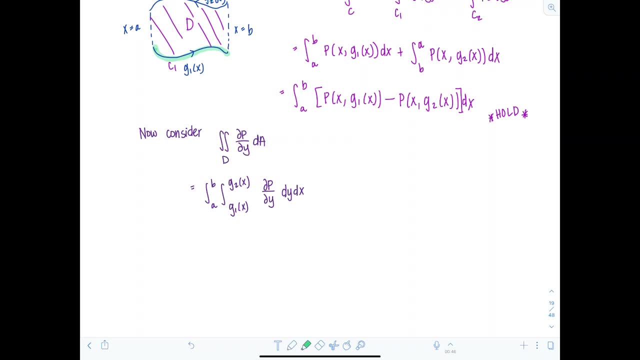 Okay, Now let's think here, Let's go ahead and anti-differentiate. If I anti-differentiate del P, del Y with respect to Y, I'm just going to get back P, right, Cool. So now I have integral from A to B, P of X, Y, evaluated from G, sub 1 of X to G, sub 2 of X, DX. 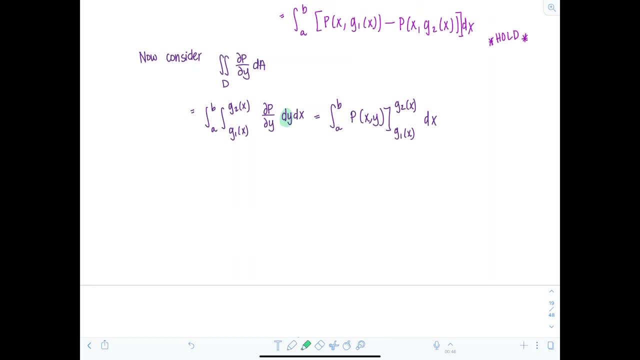 Now, where do I plug in these limits of integration? Well, I just anti-differentiated with respect to Y, So they get substituted in for Y. So now I have integral from A to B of P of X, G sub 2 of X. 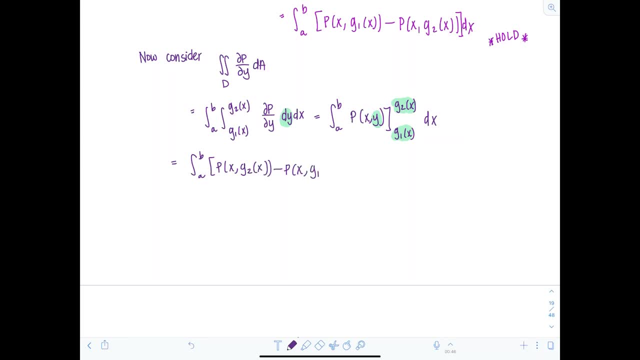 minus P of X G, sub 1 of X DX. This is exactly what we put on hold earlier. Do you notice? These are the same. So what did I just show? Therefore, we showed that the integral over the closed curve C of PDX. 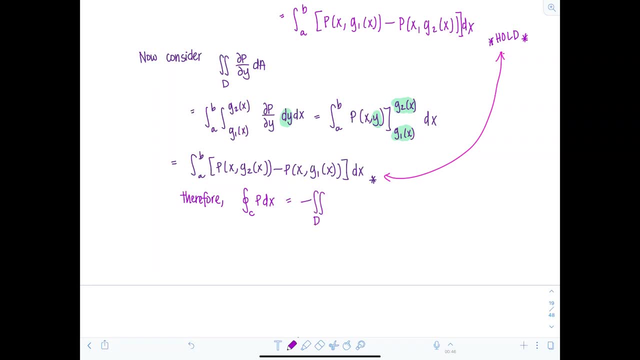 is equal to the opposite of the double integral over D, del P, del Y, DA, as desired. So that's the first half. I'm going to let you complete the second half and I'll just give you an outline of how to do it. 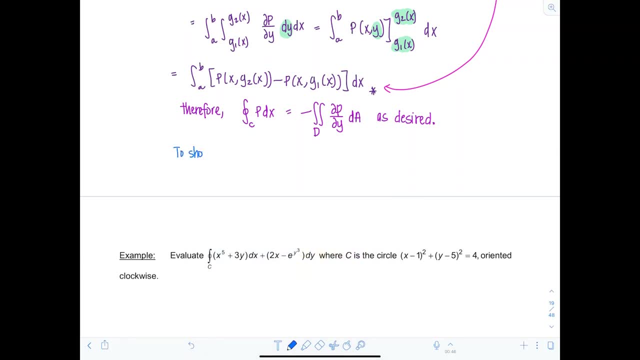 So if you want to show that the integral over the closed curve C of QDY is equal to the double integral of del Q, del X, dA, all you need to do is use a type 2 region where you would put constant limits for Y on the outside of your double integral right And you have X defined. 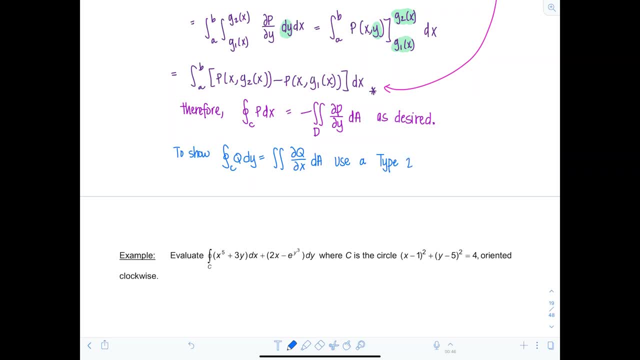 in terms of Y, bounding the region on the right and left. So you write it as a type 2 region And then you can just basically mimic the process that I have outlined up above. Okay, so I really recommend you take the time to make sure you can write out that proof properly. 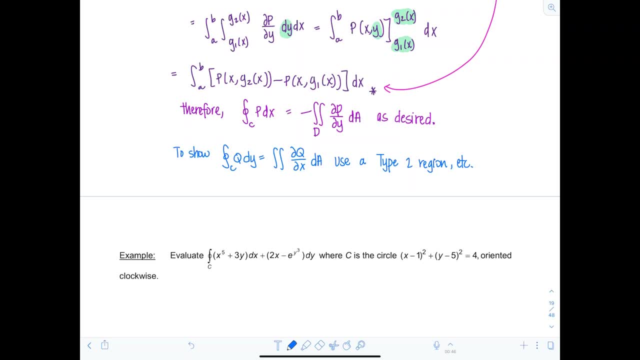 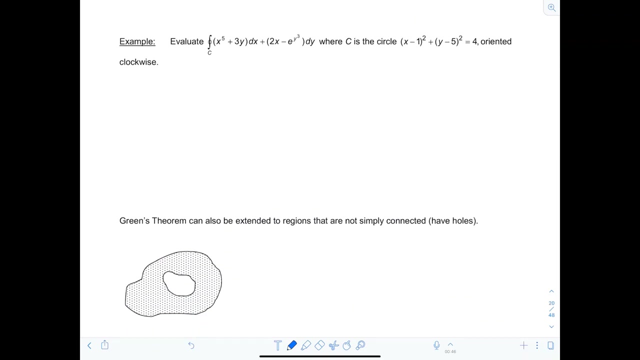 Okay, it's good for the brain, All right. so now, hopefully, you believe Green's theorem in your deepest heart of hearts, so that now we can apply it freely. Let's look at an example here. So evaluate the following integral over the closed curve C And notice: this is P, dx plus Q dy. Here's P, here's Q. 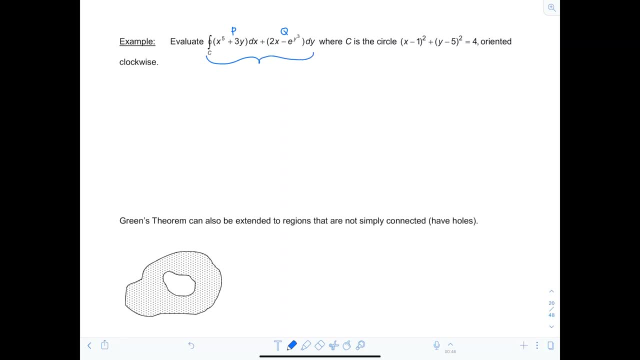 this represents work. I'm going to say it over and over and over because when we learn flux and other things, it can get confusing. So I want you to keep straight what your integral represents. And then C is the circle X minus 1. 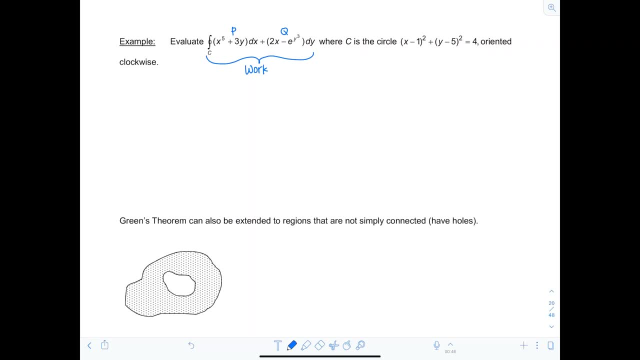 squared plus Y minus 5, squared equals 4, oriented clockwise. So that's opposite direction, right? That's the negative direction. Well, I can just take the opposite value of the integral, right. Since we're going in a non-standard orientation, we're using a negative orientation, So I have 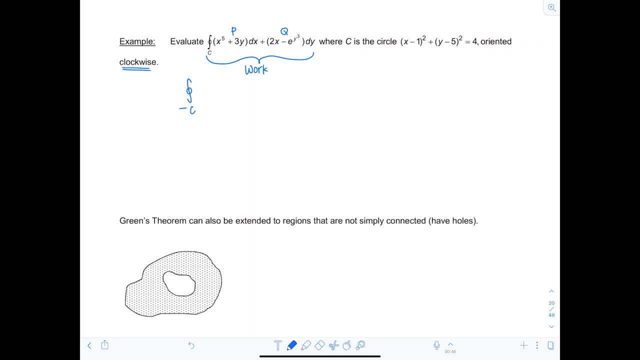 integral over the closed curve, C, I'll put opposite of C, P, dx plus Q, dy, And this is going to equal. so I'm going to use Green's theorem but I'm going to add a negative in front, Double integral over D. And remember, Green's theorem tells me I can take del, Q, del X. 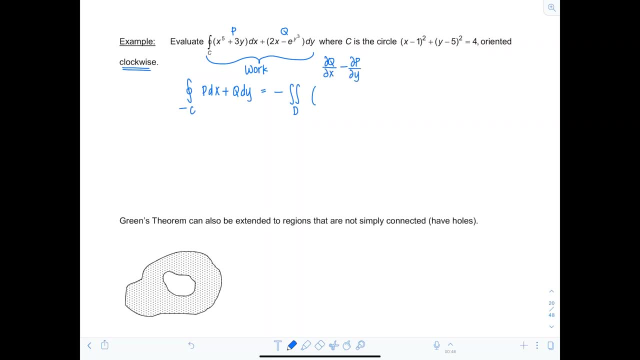 minus del P del Y. So what's del Q del X? It's 2, minus what's del P del Y? It's 3.. So that's negative 1 times another negative 1.. I have the double integral over D of D A. 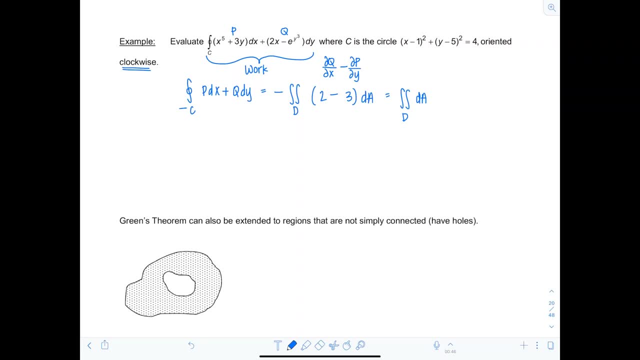 Do you remember what this represents? If you don't have a function and you just have double integral over D, D, A, this is just asking for what's the area of D? So I don't even actually need to integrate the region. This is a circle. I don't care where it's centered, I just need its. 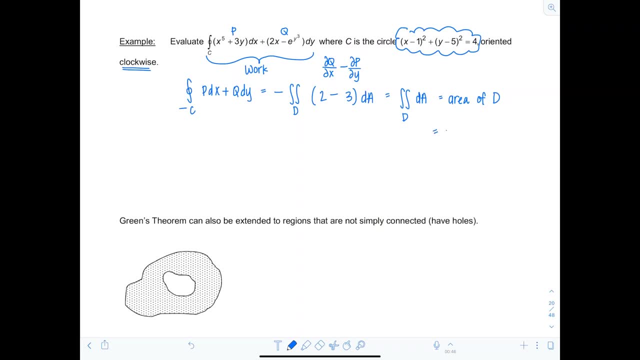 area And the area depends on the radius. pi R squared, So it's going to be pi times 2 squared times 1 squared, So 4 pi. Thank you, Green's theorem. I didn't need to come up with the. 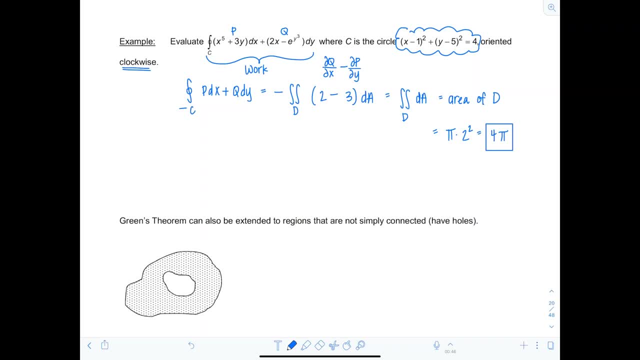 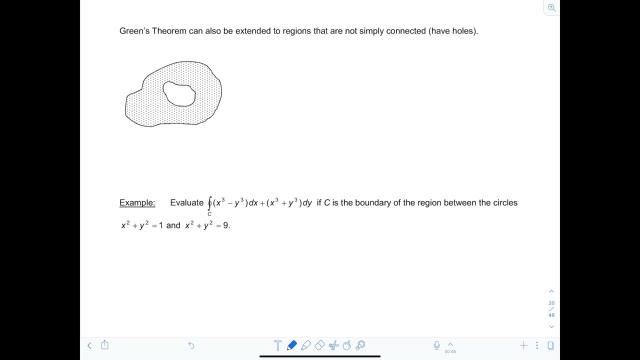 parametric representation for this circle. We could just go for it directly and it was a really easy problem. All right, Now Green's theorem can also be extended to regions that are not simply connected and that have holes. Remember, we talked about a simply connected region. You shouldn't be. 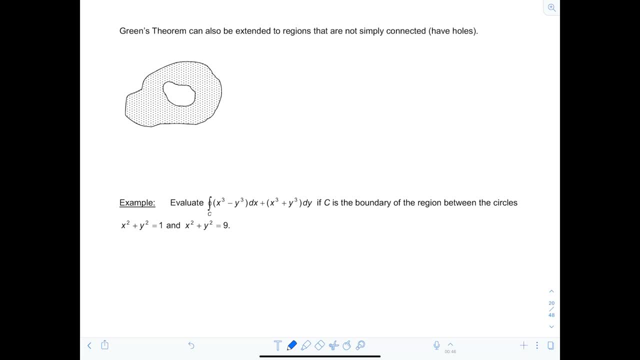 able to draw a simple closed curve within the region and contain any other points that are not in the region holes. it's not simply connected, however. in practice, all you need to do you can still use with green spam and then just subtract out the work, so subtract that. 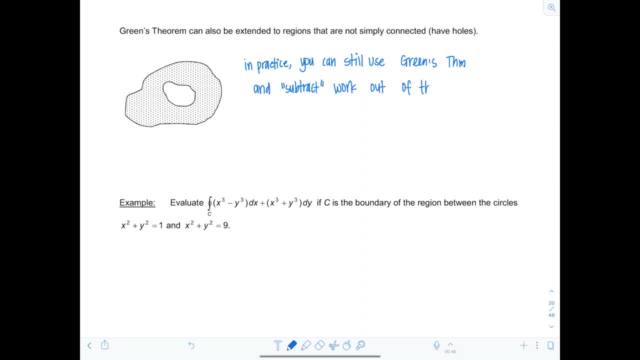 work out of the missing regions. so how would you do that? well, you would just impose a curve with negative orientation around the region where there's a hole that's missing, and then that would subtract it out. so, like here, I would impose a positive standard clock, counterclockwise orientation, right and 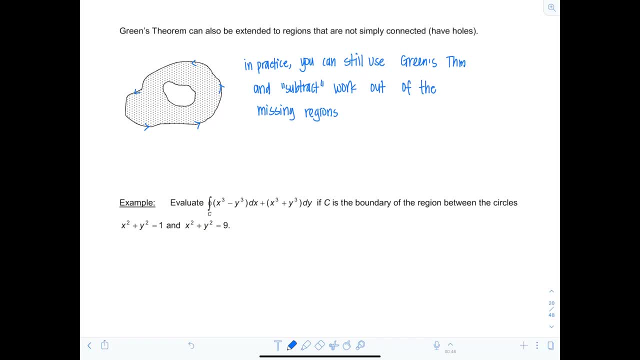 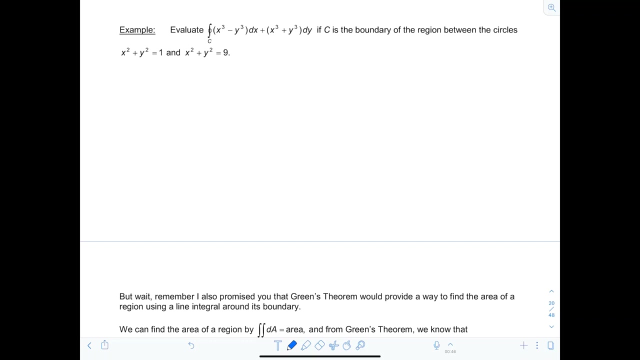 then, since I want to subtract out the work on this missing piece in the middle, then impose a standard clockwise orientation. okay, so you could just use the double integrals and subtract out that piece. let's try another example here. so evaluate the line integral over the closed curve C. I'm not going to read it. 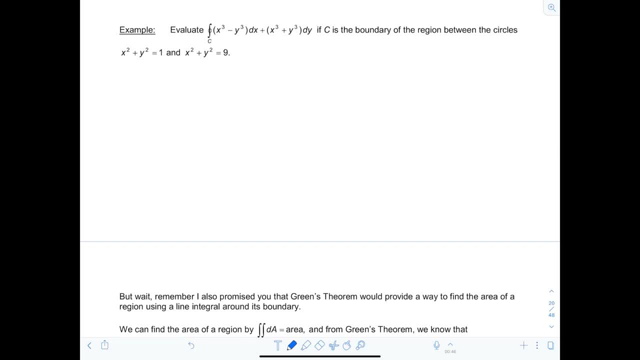 you can see it, if C is the boundary of the region between the circles, x squared plus y squared equals 1, and then x squared plus y squared equals 9. so notice here: C is the boundary of the region between these two circles. so clearly we're gonna have a hole. yes, okay. 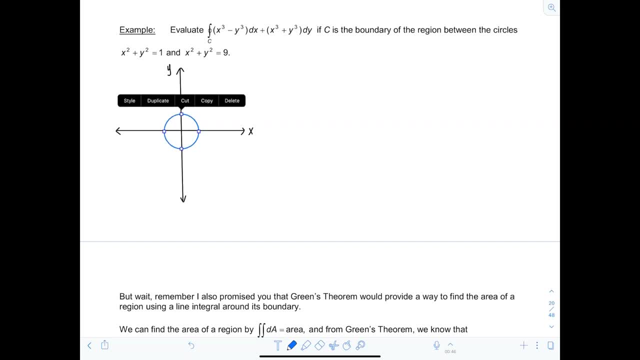 so one of them has radius 1 and then the other one has radius 3. good, so this is. I was happy where you were. okay, here's one, two, three. and my curve C is plus 8 plus x squared. so the only reason I'm calculating this is I'll need to save. it for later when I'm doing my technique right now. so I want to find the unloaded curve on my left, so I'm going to take my hide the Holderhand time and that worked well. I just wanted to make a lucky compromise and just let this work, so we're. 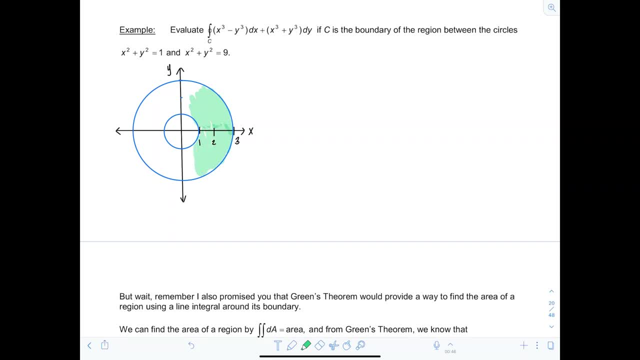 going to work on that and I were going to be looking at the two round curves, for the is the boundary of the region between these circles. okay, so there's two pieces to see. so let's think here: what would you do, well, if you were to use a line? 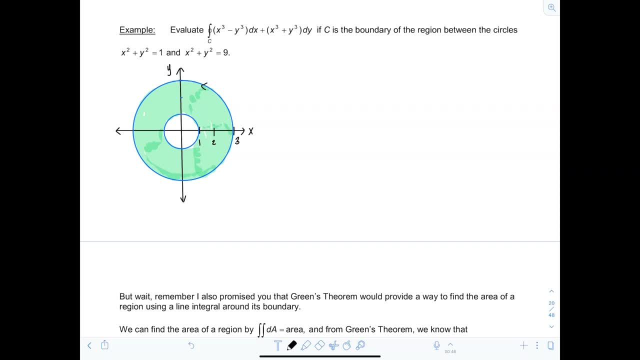 integral. right. then you would want to impose standard orientation on that outer circle, and then you would have clockwise orientation to subtract out the work on the inner circle. or you use Green's theorem and you don't even stress about it, so you have double integral over D. remember it's del, Q, del. 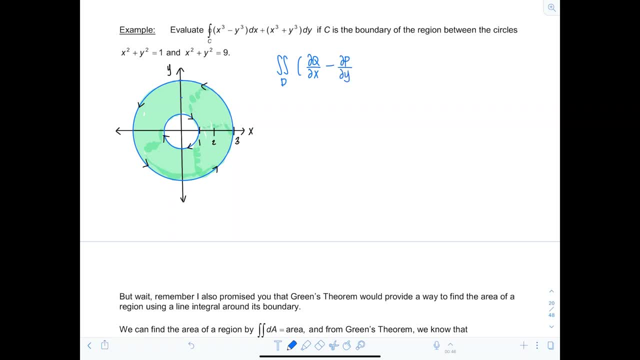 X minus del P del y. da here's P, here's Q, so double integral over D. don't commit to a coordinate system yet. until you see what it's looking like, you know what I mean. so what's del Q, del X? it's 3x squared minus del P del. 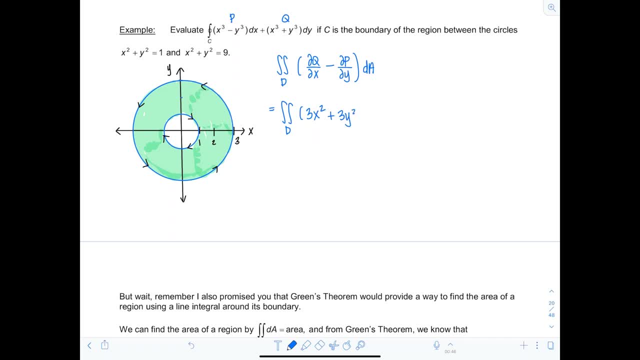 y is negative 3y squared, so this is going to be plus 3y squared. da, now you were probably suspecting we'd have to go polar. I mean, these are circles for crying out loud. and then now you see, the integrand is 3x squared plus 3y squared. 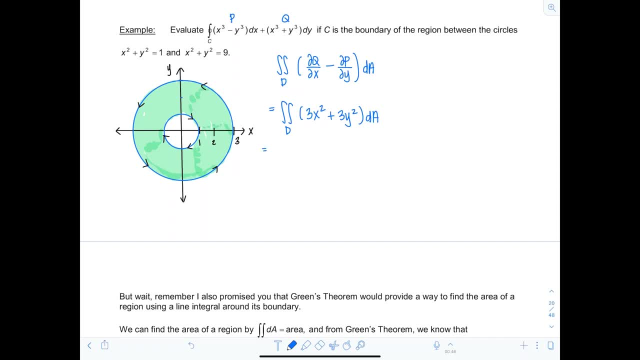 of course we're gonna go polar. so when you set it up you just account for the hole in the middle. so theta is gonna go from 0 to 2 pi, but then R is only gonna go from 1 to 3 and then, in terms of polar, 3x squared plus 3y squared, that's 3r squared, and 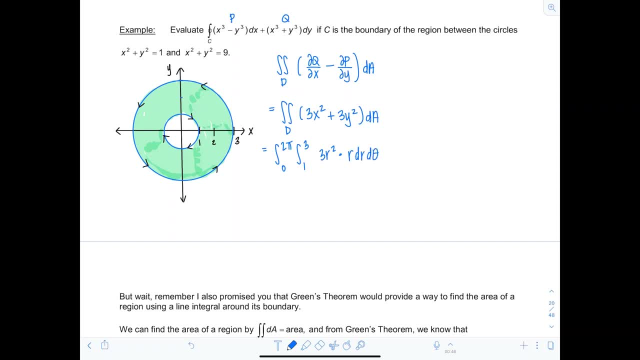 then da is gonna be R dr d theta and then this is a super nice, easy integral, right? so there's no thetas in there and here's a 3, so I can just multiply 3 and 2 pi, that's 6 pi, and then I have integral from 1 to 3: R cubed dr and. 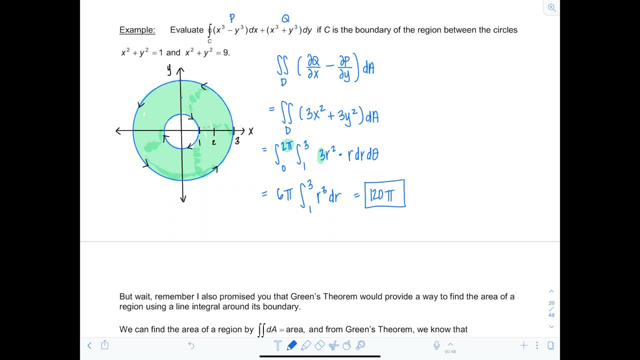 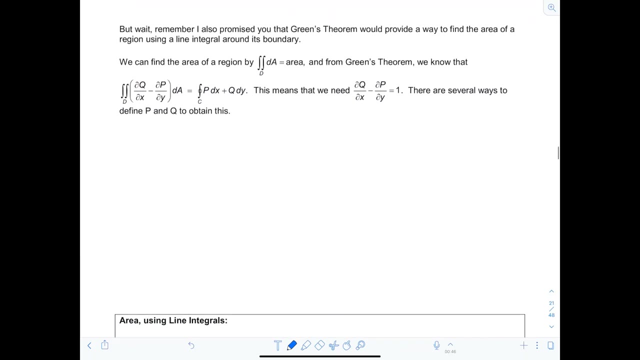 this gives us 120 pi. very good, very, very good. so how do you like Green's theorem? so far, it's pretty fun, right, and the integrals aren't too crazy. but remember, I promised you something else. I promised you that Green's theorem would provide a way to find the area of 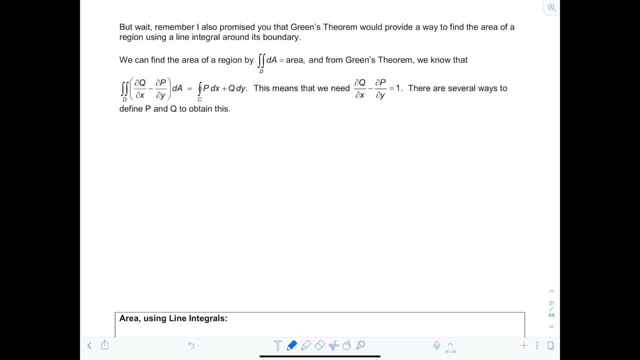 a region using a line integral around its boundary and, as we've talked about before, you can find the area of a region by evaluating a double integral of just dA. right, you use your function to just be 1, the integrand is 1. so from Green's, 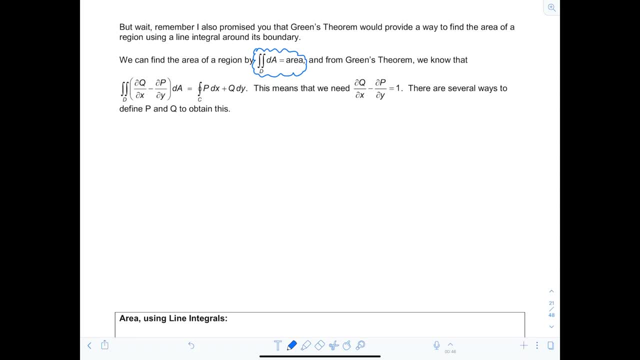 theorem. I know that the double integral over the region d of del-q, del-x minus del-p, del-y, dA is equal to the line integral over the closed curve C of pdx plus qdy. so if I want this integral to give me the area of the region that 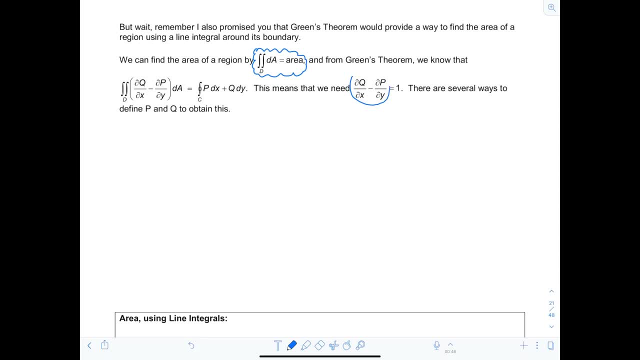 it encloses. then I need del-q, del-x minus del-p, del-y to equal 1. right, then, that way this would just be a 1.. So there's several ways to force or to make this happen. One way, you would let p equal 0,, q would equal x, and then del q, del x. 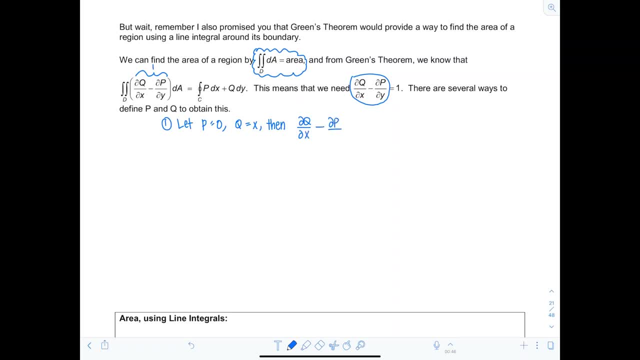 minus del p del y would be equal to 1 minus 0, which is 1.. So if you have the double integral over D of del q del x minus del p del y dA, then that would be double integral over D of dA right, Which would be the area of D, which would equal the line integral over our 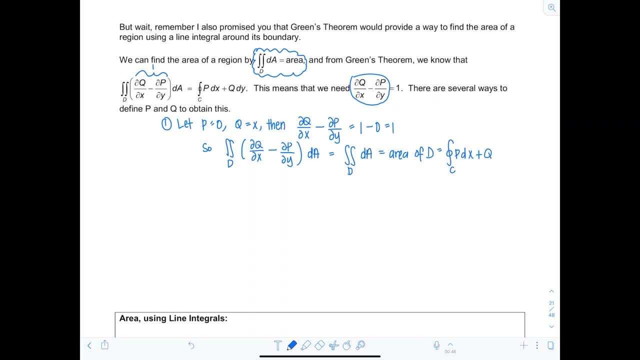 closed curve C of p, dx plus q dy. But remember we let p equal 0, right? So if we want to do this, we're going to have to put double integral over D of del q. del x, P is equal to zero. then I just have line integral over the closed curve C. Q was also. 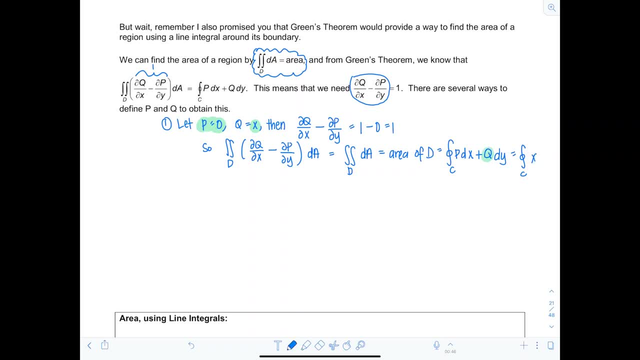 equal to X. so I just have X, D, Y, Right here. That's option one. I got more options for you. Option two: you could alternatively let P equal negative Y, Q would be zero, and then again, del Q, del X minus del P del Y would equal zero minus negative one, which. 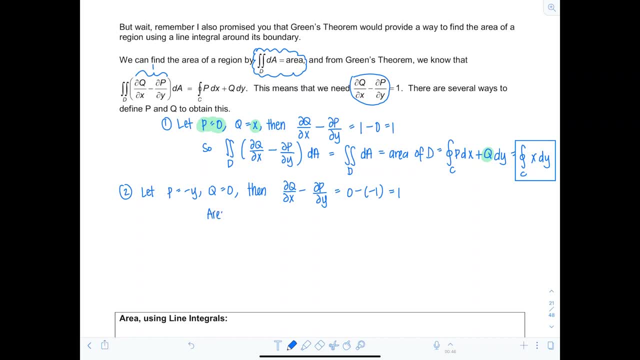 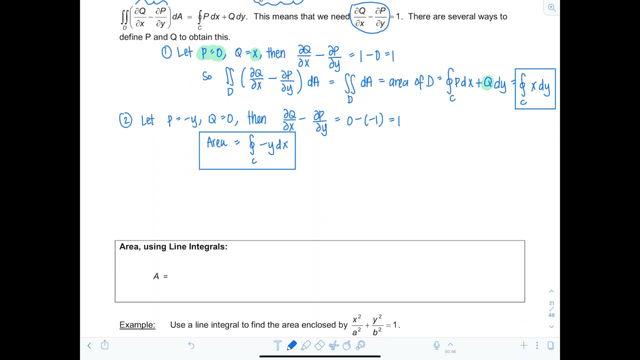 is one. So in that case the area would equal line integral over closed curve C of negative Y DX. Good, I like having options, don't you? Third option: you can combine the first two together. Combined, meaning, you add equations one and two. Well, if I add them together, then I. 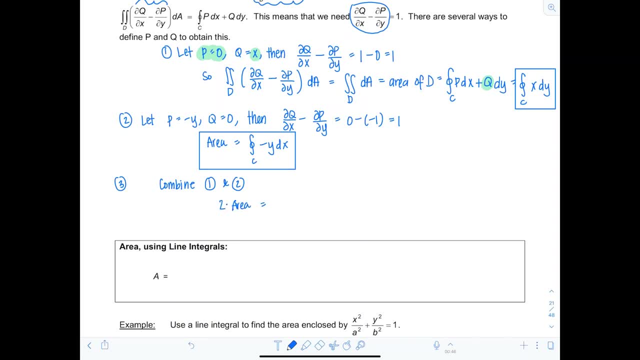 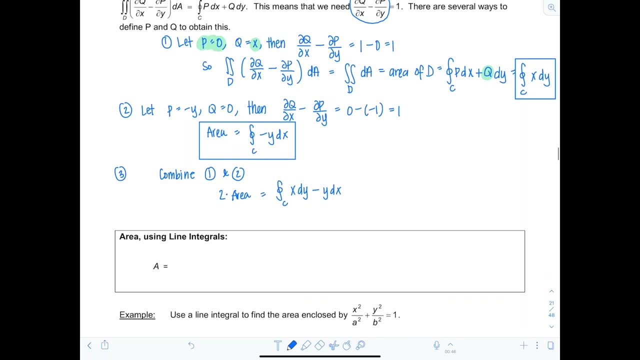 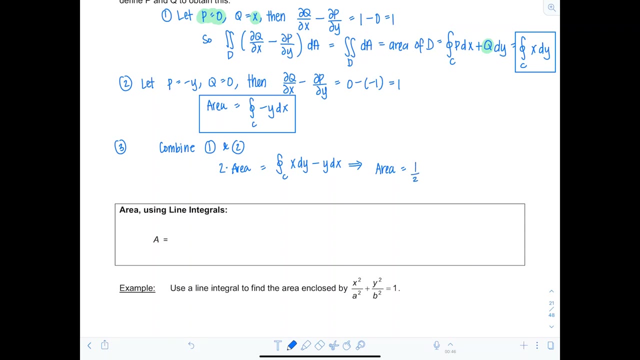 have two times the area equals line integral over c of x, dy minus y dx. So if you just want the area you would divide by two. So area would equal one half times the line integral over the closed curve c of x, dy minus y dx. All right, which one to use, It depends on the problem. Sometimes one is more. 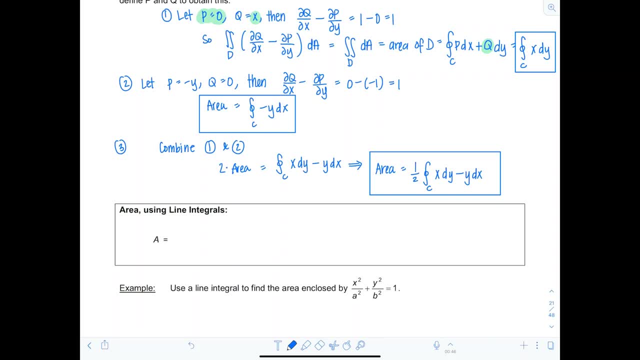 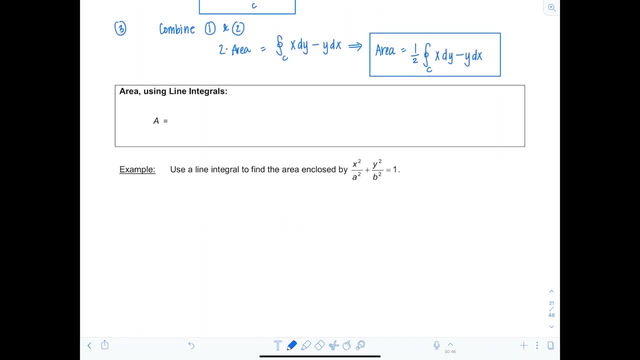 friendly to work with than another, So we'll do some examples. Okay, good So area using line integrals. I'll just summarize the three options So you can either integrate over the closed curve c, x dy, or negative y dx, or one half both of them added together: right x dy minus y dx. We'll use this last result for the. 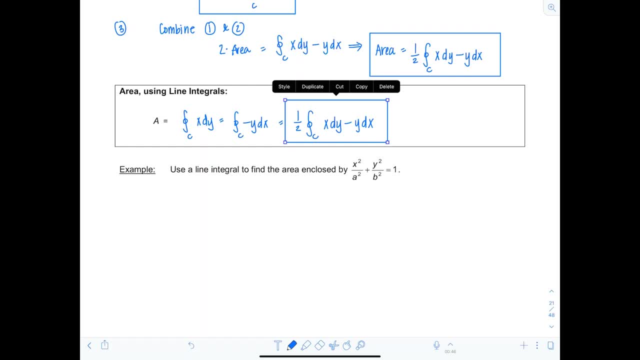 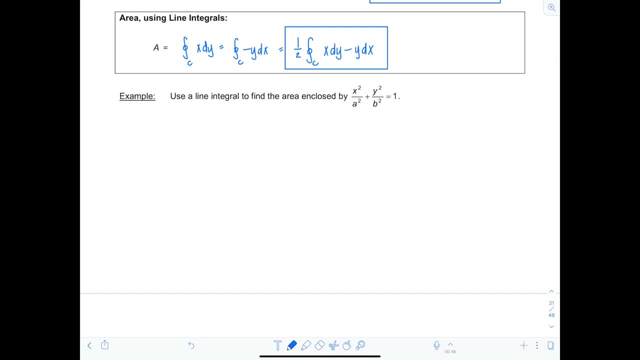 following problem and you'll see why in a second. It just makes an easier integral. Use a line integral to find the area enclosed by x squared over a squared plus y squared over b squared equals one. Do you know what this is? the graph of? That's right, It's. 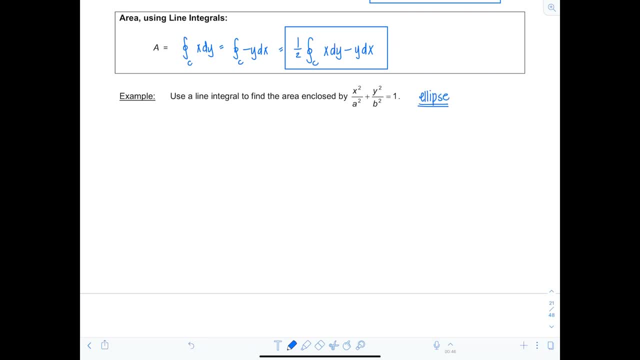 an ellipse, Do you know? there's a formula for the area of an ellipse and it comes from here, So we're going to use a line integral, meaning I have to parameterize the curve that traces out this ellipse. Do you know what it is? So we've done several examples like this. 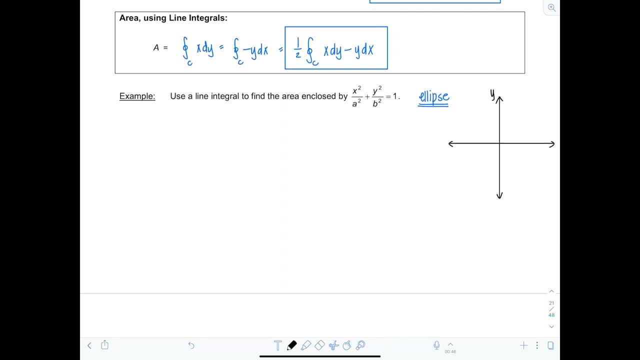 Here's the y-axis, Here's the x-axis, and we have some sort of ellipse centered at the origin. Oh no, I didn't want it to be a circle. Okay, now it knows what I want. sort of It's too lopsided, I'm just going to draw it myself. 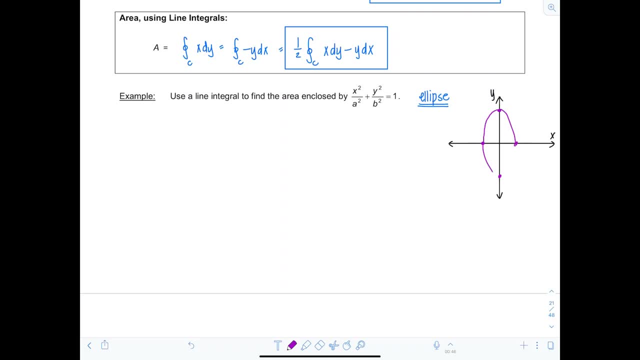 Okay, there we go. So this is at a zero, this is zero b negative a zero, zero negative b. So if I'm going to parametrize the curve that encloses this region, here x would equal a cosine t, y would equal b sine t, and then I need d x and d y. So d x would be negative a sine t, dt d y would. 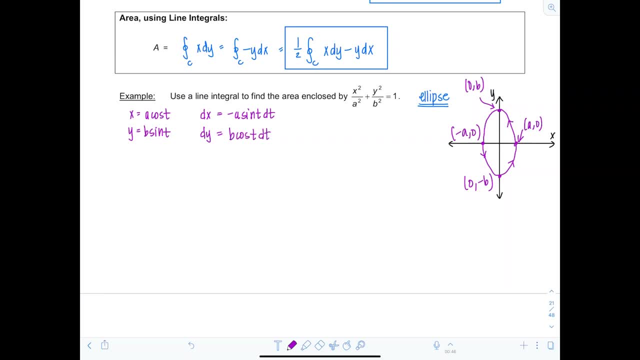 be b cosine t dt vary from 0 to 2 pi. Okay, very nice. So let's go ahead, substitute everything into the area formula And, like I said, I'm using that third version with both dy and dx in it. So area is: 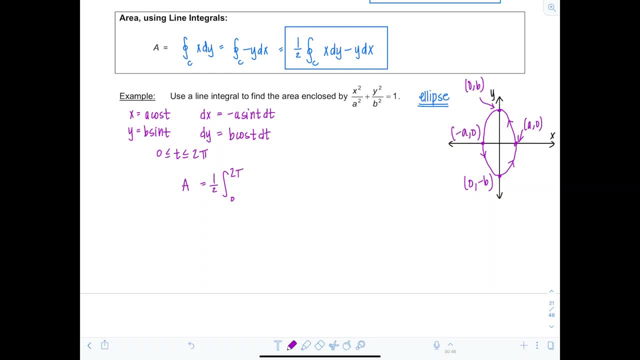 going to equal 1 half times the integral from 0 to 2 pi. So I have x dy. So that's going to be a cosine t. dy is b cosine t dt minus y dx. y is b sine t and then dx is negative, a sine t dt. 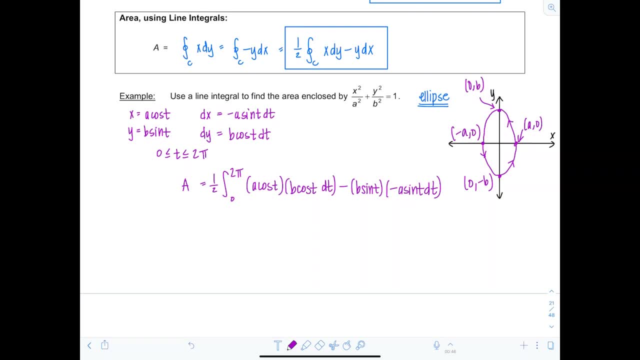 And I wanted to use this version of the integral because now I can use a nice trig identity here. see, Because I have ab cosine squared t, and then I have ab cosine squared t, and then I have ab cosine squared t, and then I have ab cosine squared t. 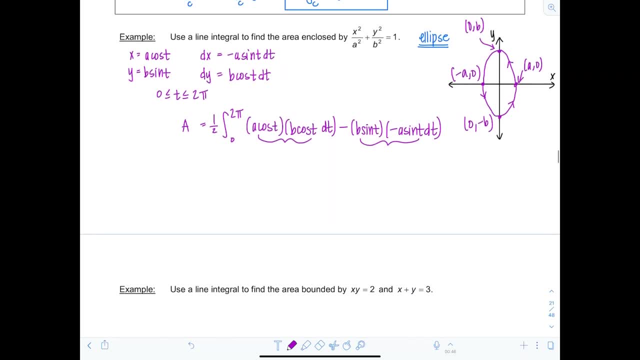 sine squared t. So that's just going to give me ab. So now we have 1 half integral from 0 to 2 pi ab dt. Well, there's no t's, so I'm just going to multiply by 2 pi. So I have 1 half. 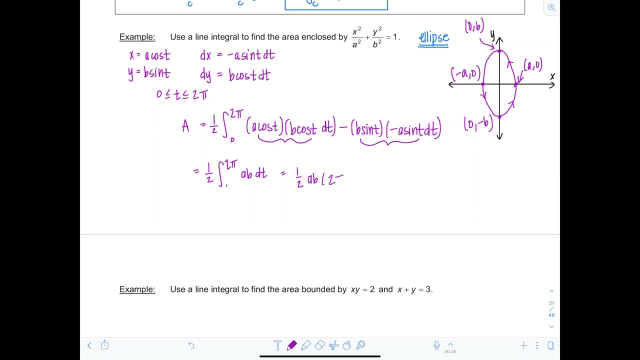 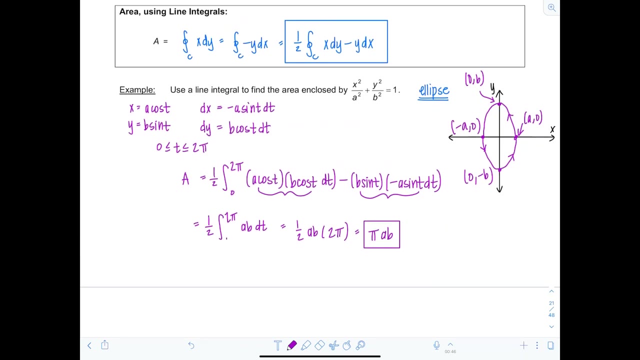 ab times 2 pi, which gives me pi times ab. Voila. So that is the area of an ellipse. And you guys did you notice something super exciting? In a circle a is equal to b, So in a circle you would have pi times a times a or pi a squared. 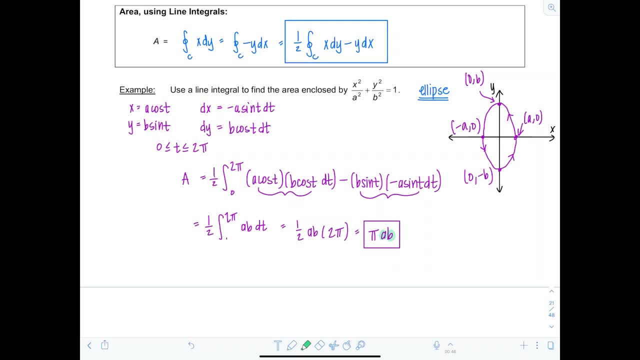 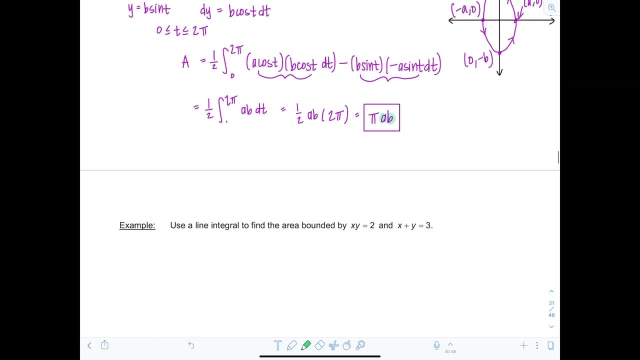 which is pi times the radius squared. Oh, my goodness, it's all coming together. All right, let's do one more, And then that's it for this lesson. So use a line integral to find the area bounded by x. y equals 2, and x plus y equals 3.. 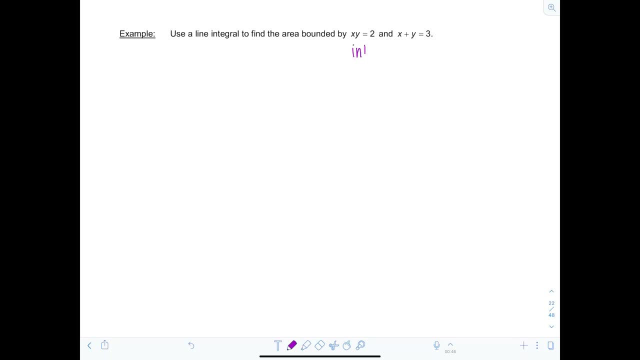 Okay, so first let's figure out where they intersect. Okay, x, y equals 2, that's the same as y equals 2 over x. And then x plus y equals 3, I'm just going to substitute in for y, 2 over x. Okay, let's multiply the equation through by x. 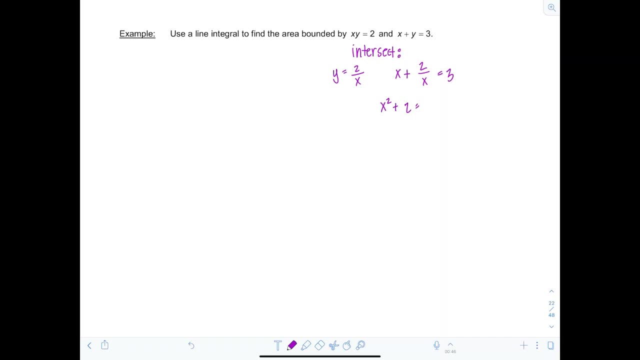 clear out the variables from the denominator. So x squared plus 2, equals 3x. So I have x squared minus 3x plus 2 is 0.. So you can factor that That means they intersect when x is 2 and 1.. So if x is 2, y is going to be 1.. So at 2, 1.. And when x is 1,. 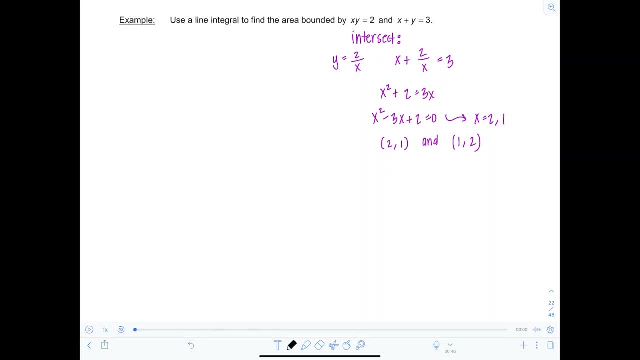 y is 2.. So that's where they intersect. Okay, so let's graph these. We're going to stay in the first quadrant. So here's my y-axis, Here's the x-axis, And 1,, 2, 3.. 1,, 2,, 3.. Let's draw our line. It has x and y intercepts at 0,. 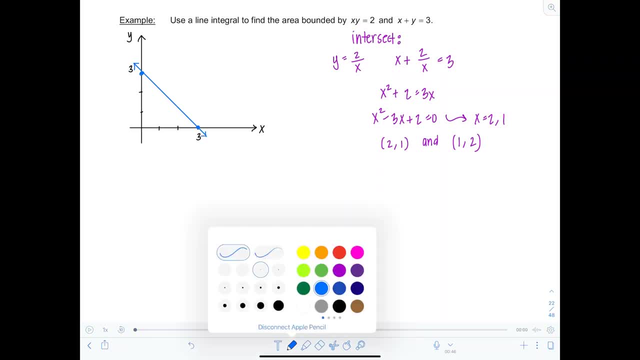 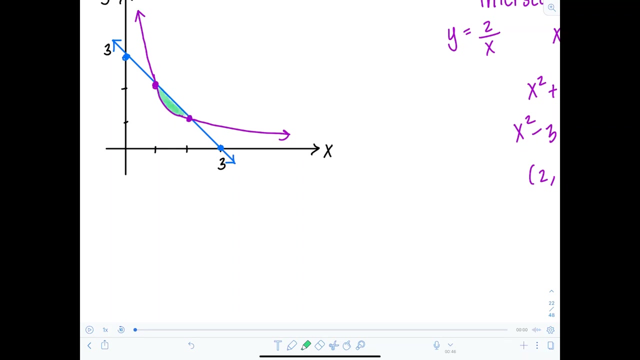 3, 3, 0. And then it intersects with the curve at 1, 2, and 2, 1.. So the region isn't going to be really big that they contain. It's going to be this little sliver in here. Okay, All right. Well, if we're going to use a, 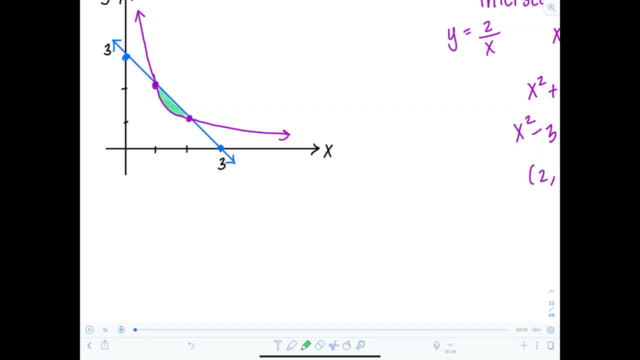 line integral. to find the area bounded by it, I need to make sure that first I bound the area using a closed curve that has standard orientation, So counterclockwise. So if you're walking on the curve, the region needs to be on your left. So let's think about it. 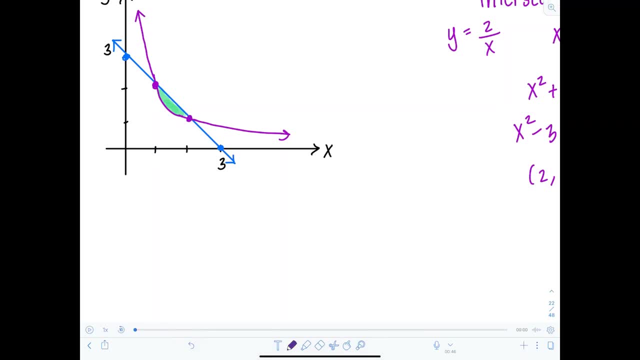 That means I need one curve going this way and then the other one's going to go down. Yes, Okay, So let's come up with our parametric representation. So curve 1 needs to go from the point 2, 1 to 1, 2.. 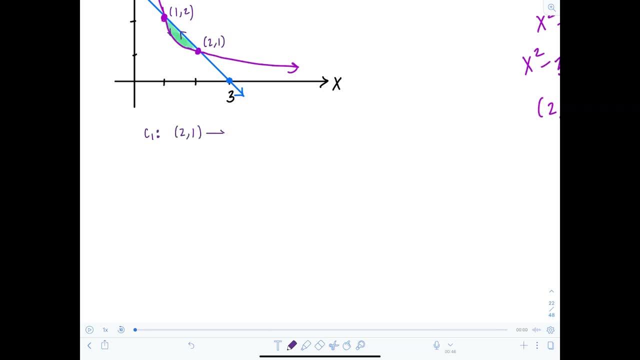 Do you agree? We're going to go from 2, 1 to 1, 2.. Okay, Our direction vector would have components. Just think back to when we came up with a parametric representation for a line segment. Yes, So it's okay that we're just in two space. 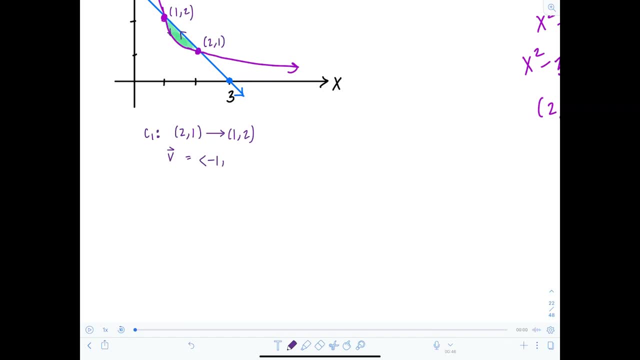 It's cool. So my direction vector would have components negative, 1, 1.. And remember you use the starting point, So use 2, 1 as your p-naught. So then x would be 2 minus t, Y would be 1 plus t. And then remember what do you have to do to t so that you only get that. 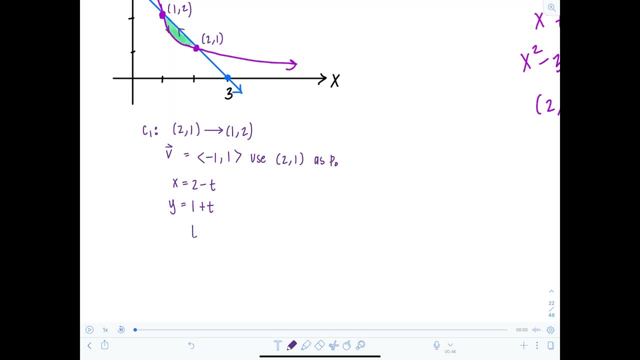 portion of the line segment from 2, 1 to 1, 2?? That's right. You restrict t between 0 and 1.. Okay, And then dx is negative, dt, dy is dt, And that one's ready to roll. 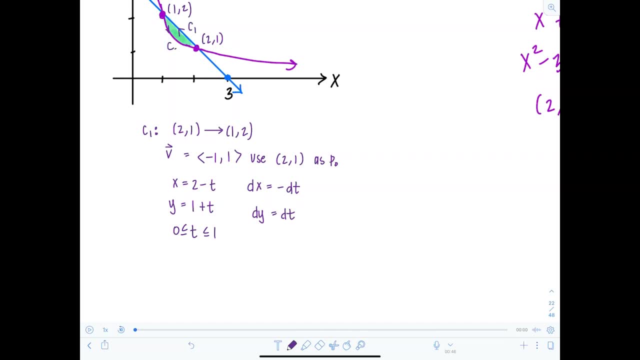 So this is for curve 1, right here. Now this guy is curve 2.. Curve 2, that's no big deal. Curve 2 comes from: y equals 2 over x, And x is going to range from 1 to 2.. So I can just let x equal t. 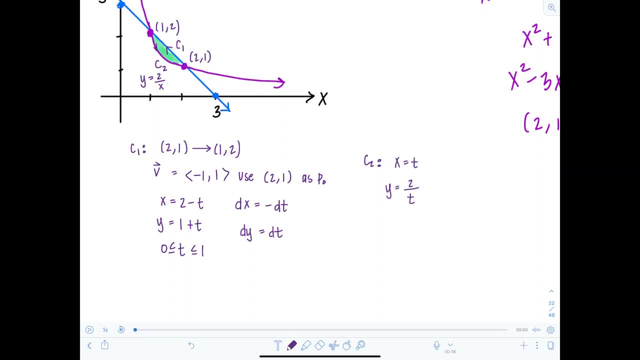 And then y would be 2 divided by t, And then I'm just going to let t vary from 1 to 2.. Okay, So dx is dt, dy is going to be negative, 2 over t squared dt, But now it looks like we're ready to roll. Yes, Okay, Now we have three. 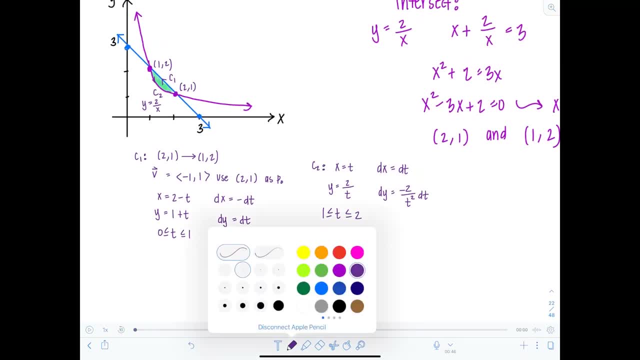 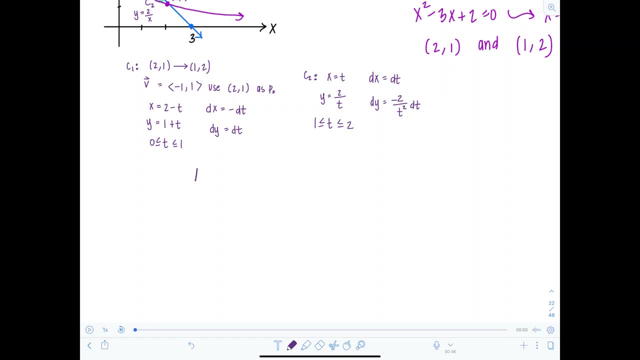 versions of the formula that we could use for area. I'll let you pick whatever you want. Just to spice things up, since we used the third version, I'll use the first one today. So area it's going to equal line integral over c1 of x dy plus line integral over c2 of x dy. 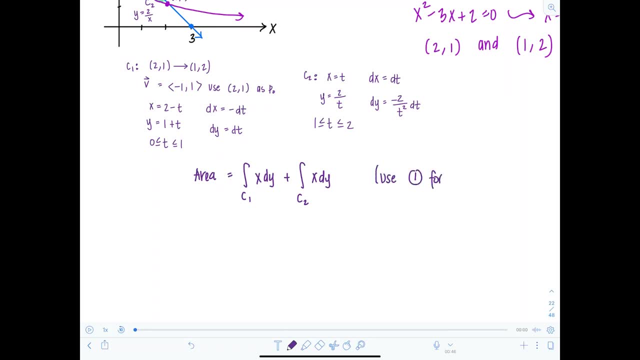 So I'm using that first formula. You know, I liked the third one for the last problem because we have those cosine squared t and sine squared t in there. that only arose when I mixed the dx and the dy, Otherwise it doesn't really help you out. Okay, Here we go. So on the first curve. 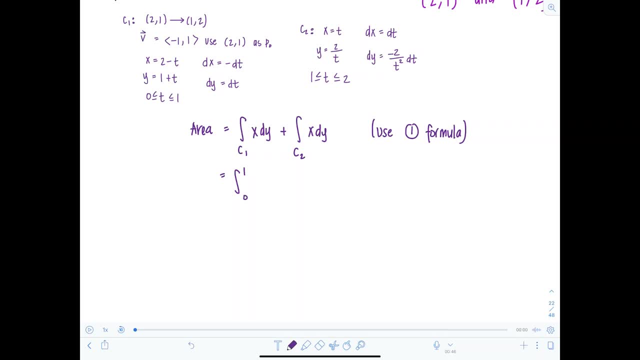 our limits are going to be from 0 to 1.. And then we're going to have a line integral over c1 of x, dy 0 to 1.. And then x is 2 minus t, dy is dt Plus. on the second curve, t limits are going to be: 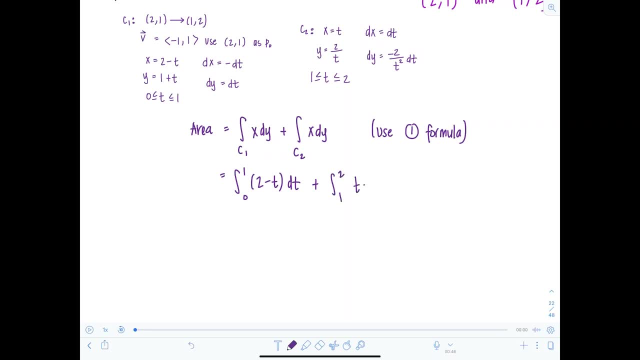 from 1 to 2.. x is t, dy is negative. 2 over t squared dt. All right, Very good, Then from here we will have 2t minus 1, half t squared, Evaluated from 0 to 1.. Plus, let's see, this is going to be negative 2. natural log Always put. 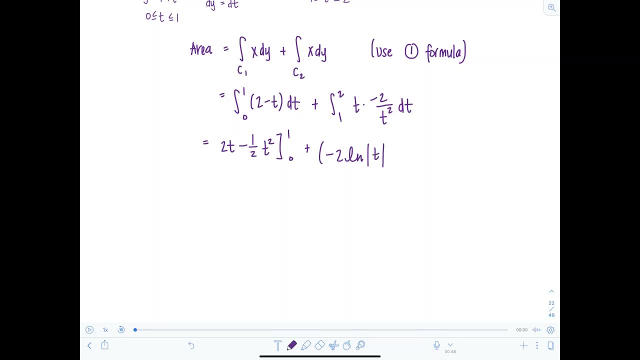 the absolute value, while you have a variable within the argument there. So absolute value of t evaluated from 1 to 2.. Then now I can substitute in my limits of integration. I have 2 minus 1, half minus 0. Minus, let's see here, 2 ln. Now I can drop the absolute value, right.